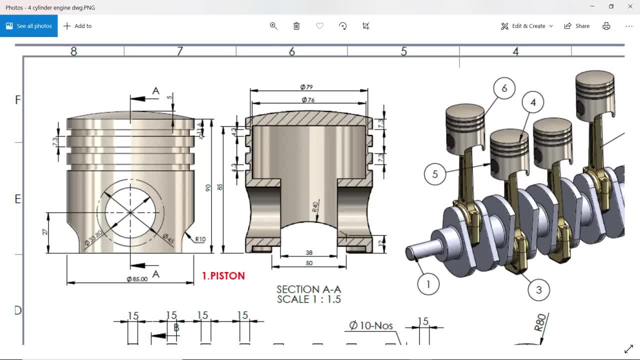 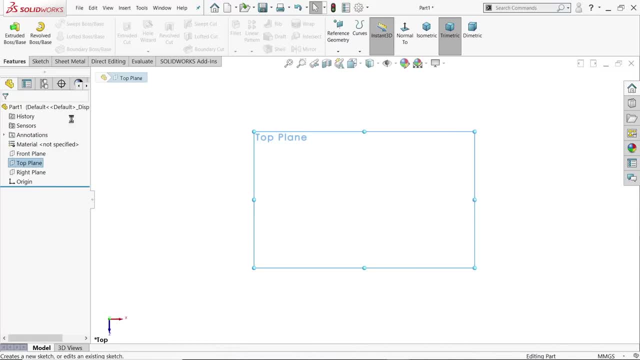 If we are going to make 3 number of things. so we need pattern 11.6 dimension. Let's do this Top plane Sketch And here I will make a circle, 85 mm. Now go to feature and choose extruded boss base and this one we will extrude up to 90 mm. 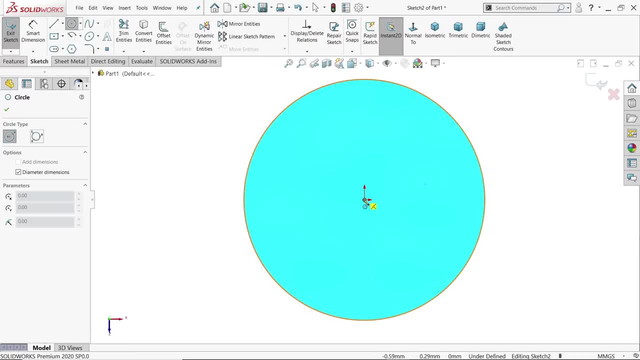 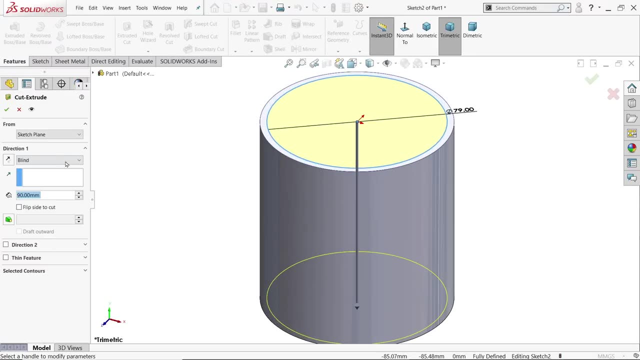 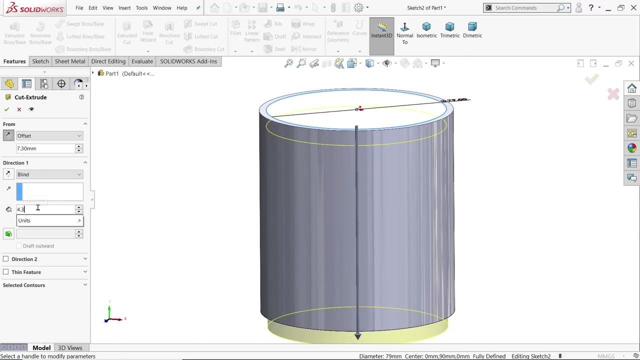 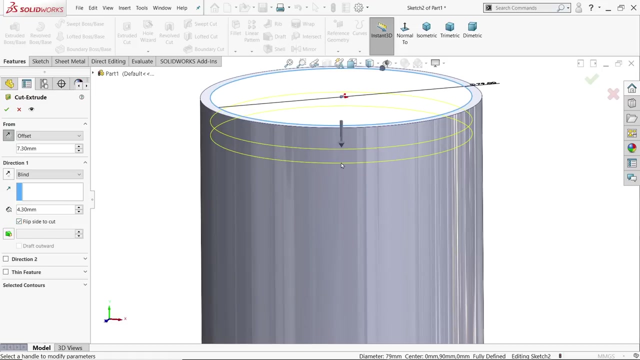 Now we want to cut piston ring. So piston ring diameter is 79.. Extruded, cut Now. we will first choose offset: 7.3 mm. reverse direction from here Blind and 4.3 mm- See Here. select flip side to cut, otherwise it will cut from inside. 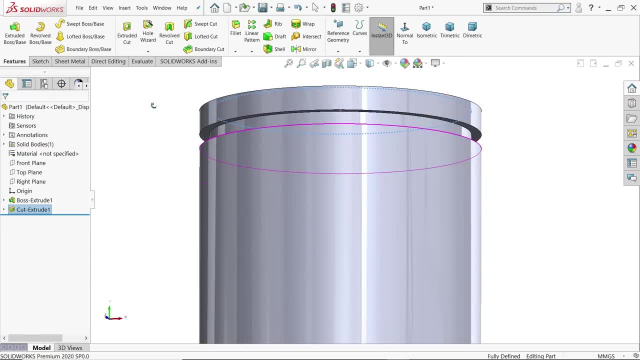 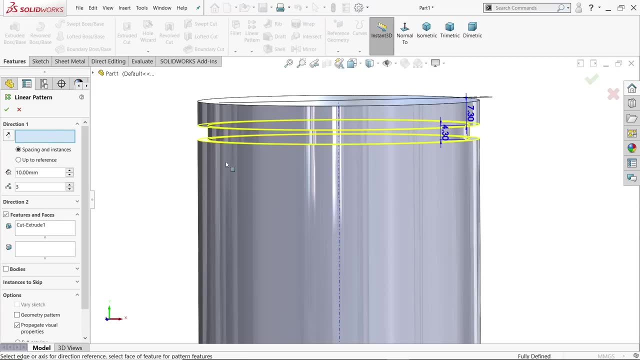 Make sure it is checked. flip side to cut. Look Show here temporary axis- Linear pattern. I will choose temporary axis And the distance it is 7.3 mm plus 4.3 mm And we need 3 number of patterns. 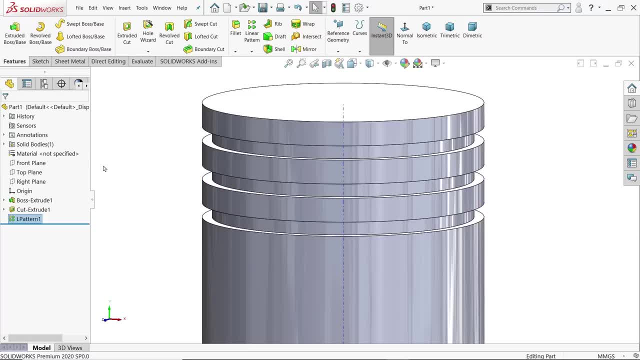 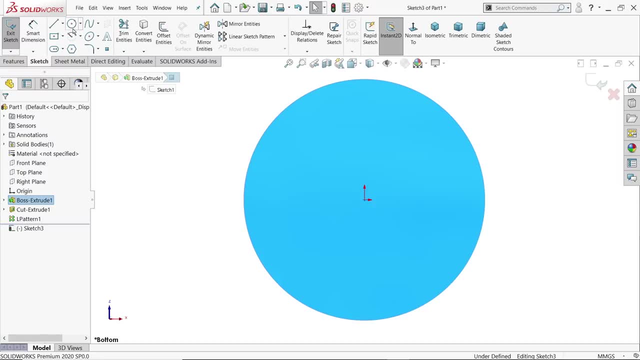 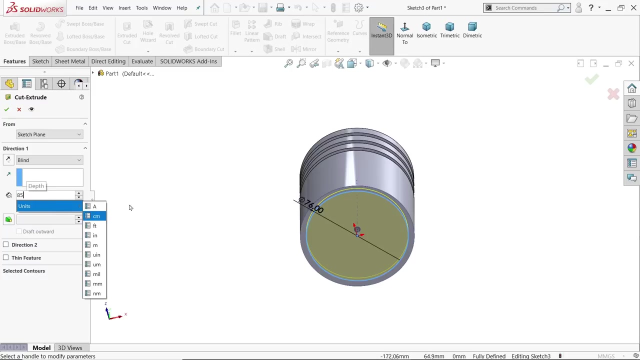 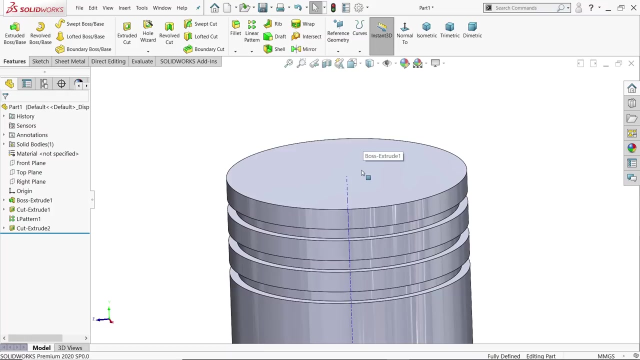 Say ok, Now. look Now inside there is a hole and the hole diameter is 76.. Extruded, cut And this cut out inside up to 85 mm. I will show you in dimension. Now let's make here dome shape. So go to insert feature and here you will find option dome. 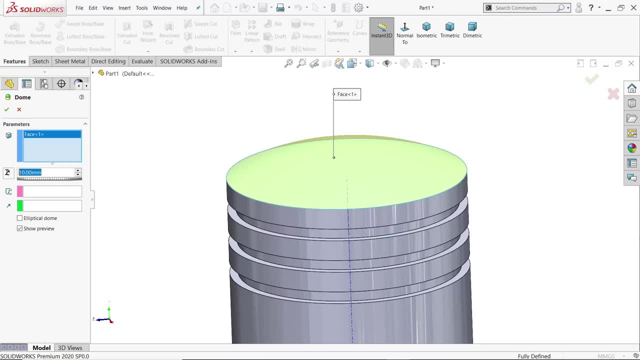 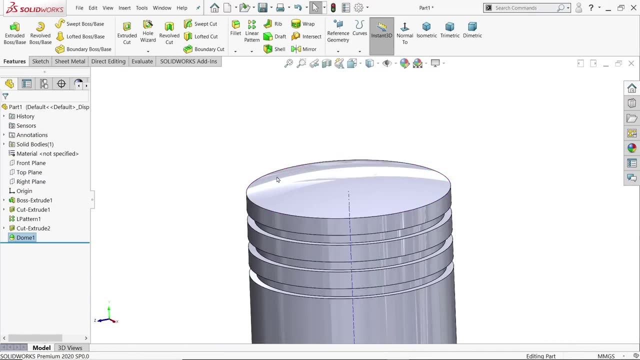 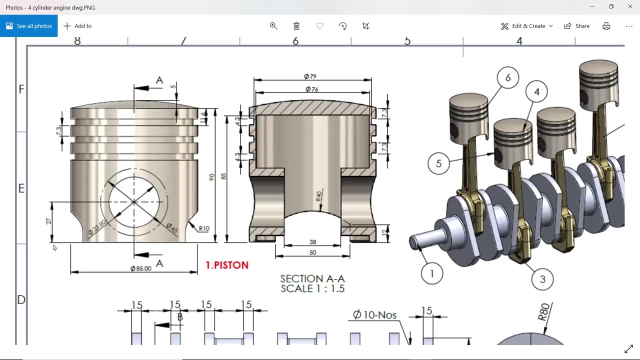 I will select this face Now. here I will make the distance 5 mm. You will see the preview. Look. Let's hide temporary axis. Now let's make this hole 27. distance from bottom: 33.8 mm. This is through out hole. 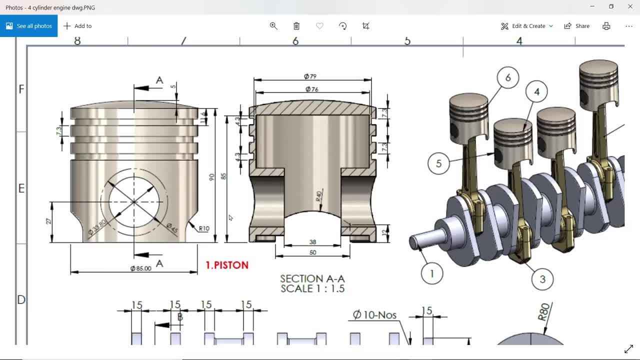 Then there is inside one extruded body and that is 45 outer diameter. See, you will see from inside. And 38 mm distance means we will, If we choose center distance. So 9 mm, we will make 19 mm, we will make offset. 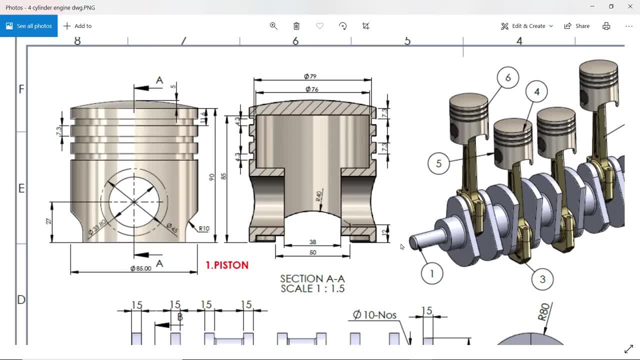 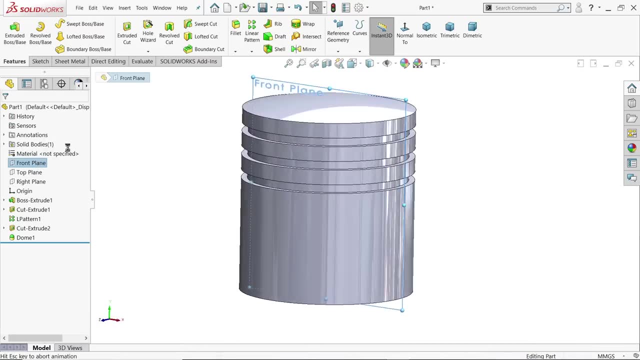 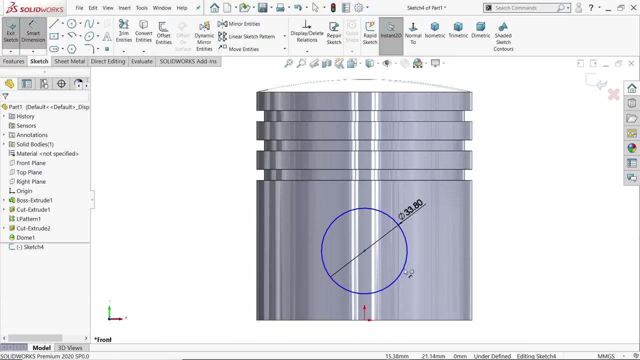 There is one more cut out. See here R 40.. 12 mm. 50. this cut out dimensions. So I will show you how I will choose front plane Sketch. This is 33.8 mm. Distance from bottom is 27 mm. 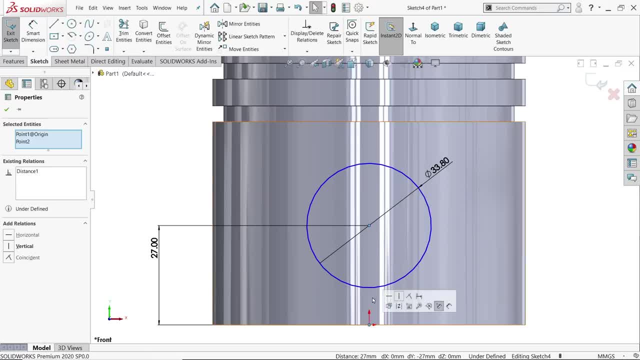 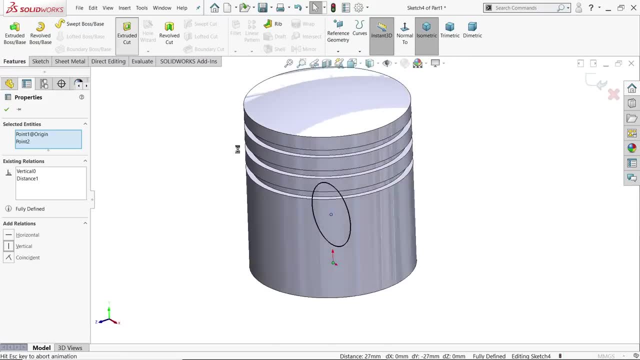 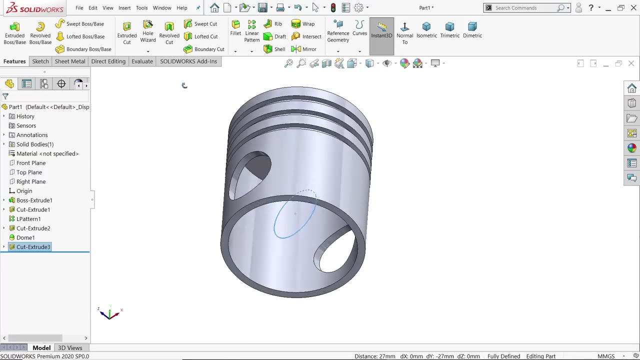 Now still not defined. So do one thing: Make one constraint relation, Select both Vertical See Feature and choose extruded cut. Now here we need to make cut through all. both Say yes, Look Now again what we will do. 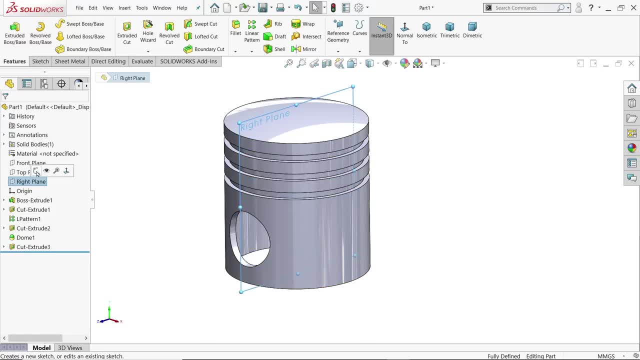 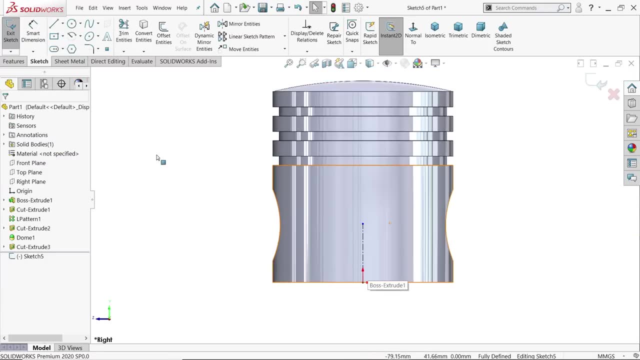 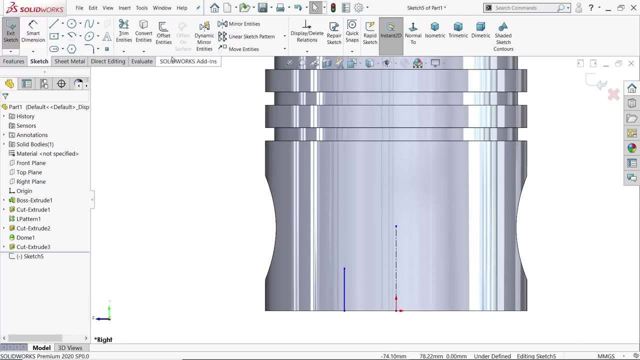 Ok, Let's cut first right plane. Let's draw one center line. Now here I will draw line. Ok, Let's select both line Mirror entity. Now here I will choose 3 point arc And I am going to connect. 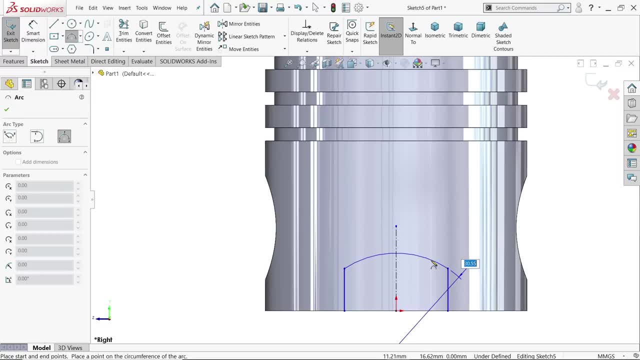 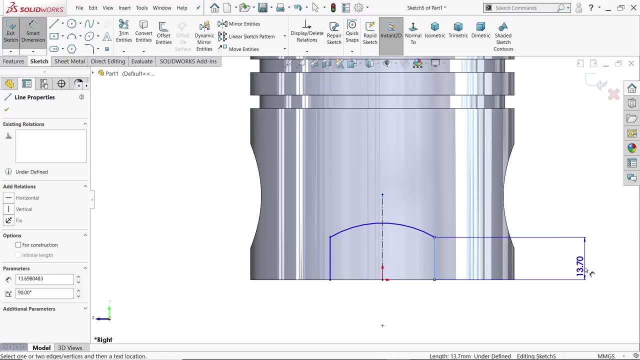 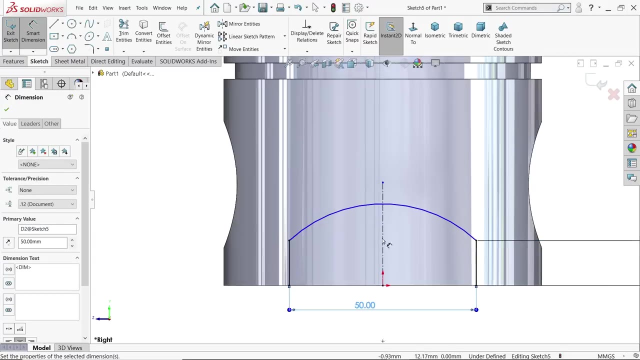 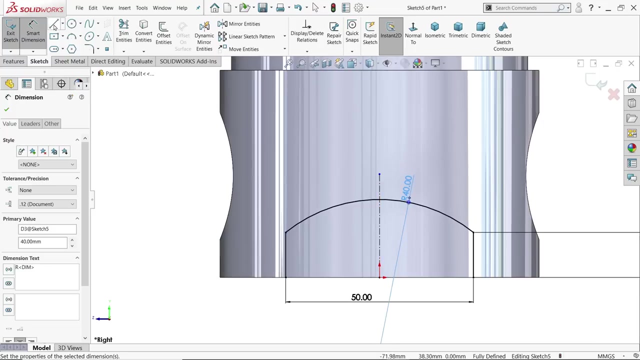 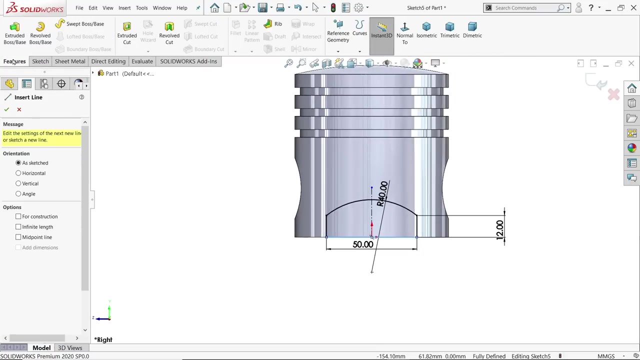 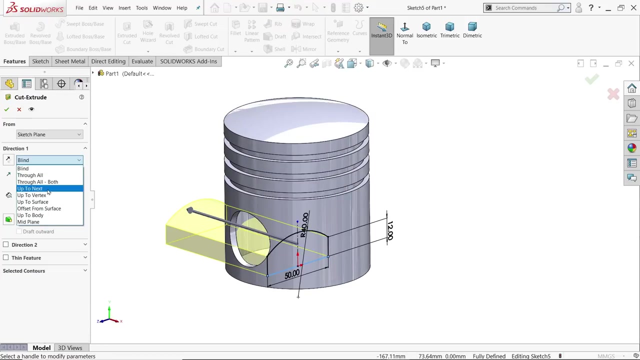 That's it Now. this length 12 mm, 50 mm And this radius 40 mm. Ok, Now let's close this one Extruded, cut, Keep, end. condition Us Both side. We want to cut both side. 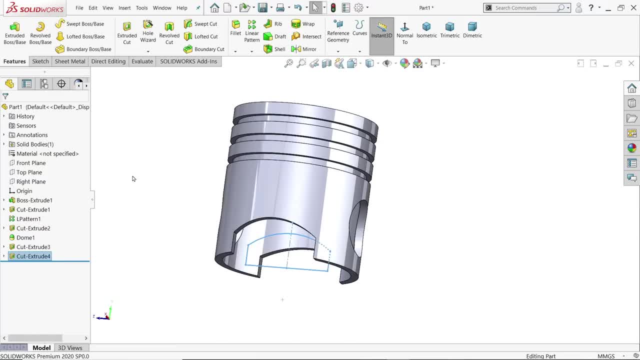 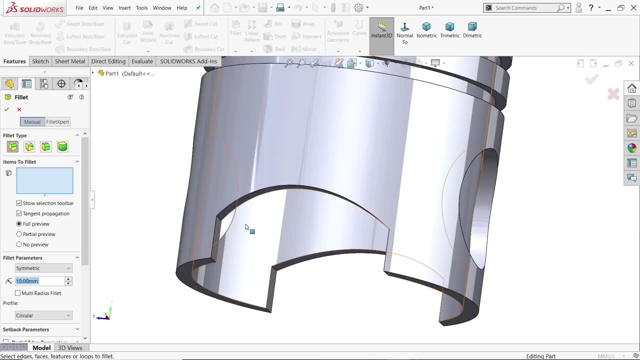 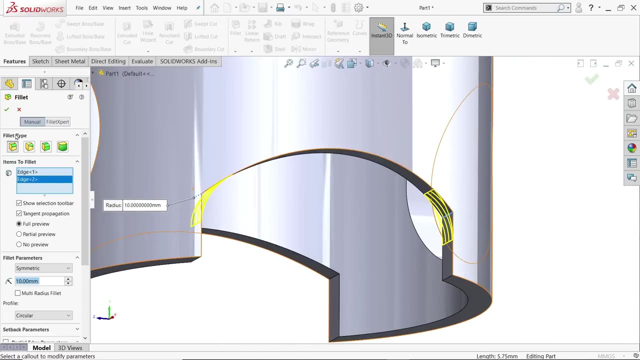 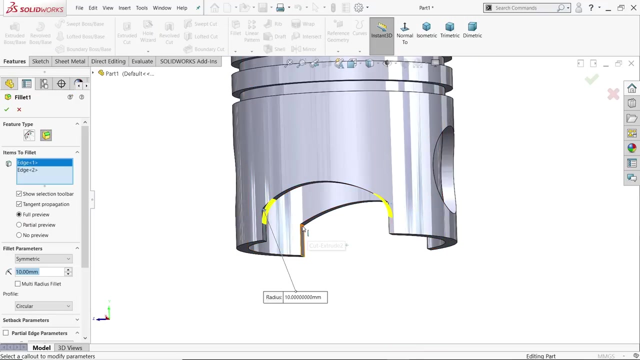 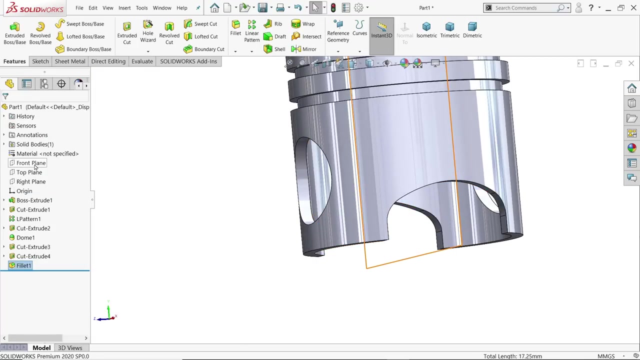 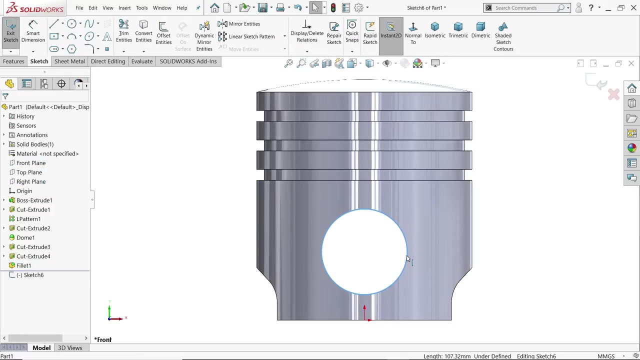 Say: ok, Now let's make here fillet 10 mm Both side. Ok, Just edit And add this: Two edges also. Now, Here I am going to choose Front plane Sketch. I will choose this circle. 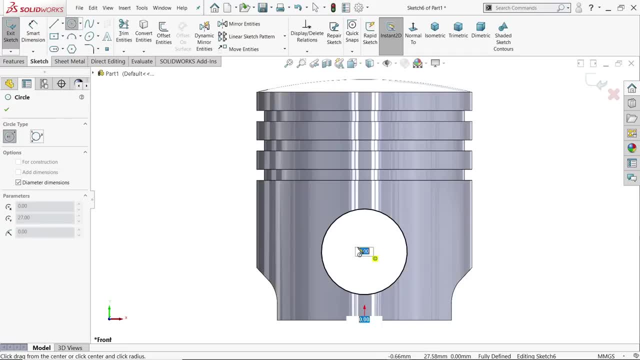 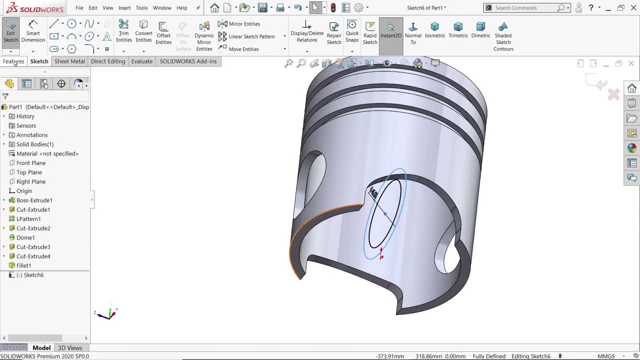 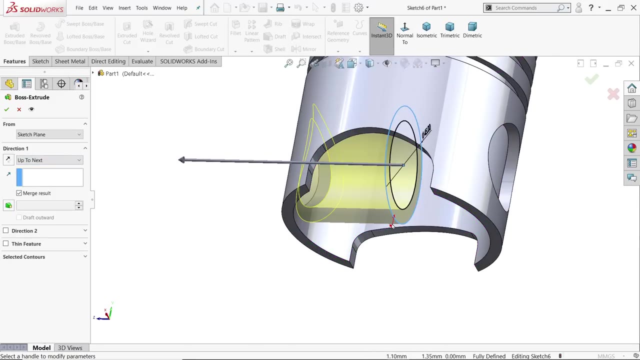 Convert entities, Then again, I will choose one more circle, And this is 45 mm. Ok, Now if you see inside, Look, Extrude. We want to extrude up to next, But Here is a catch: We need a gap 38.. 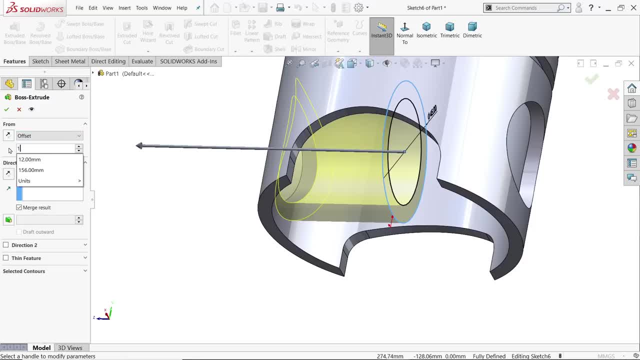 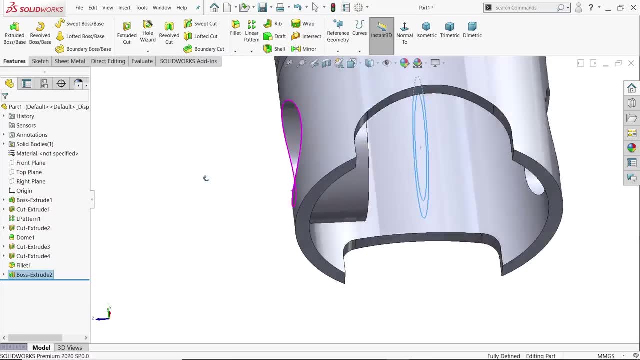 So we will make half of this Set 19 mm. Look. The half distance is created. Say yes, Look Mirror. I will choose Front plane And feature to mirror. This is here Extruded boss base Two selected. 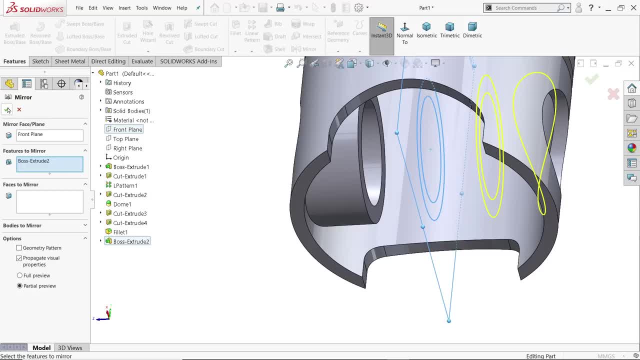 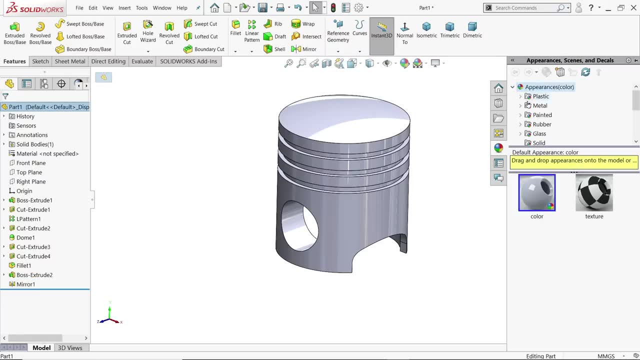 Look, This is how it's mirror. Now let's save this Metal. This is here. Extrude Boss: base Two selected. Look This is how it's mirror. Now let's save this Metal. This is here. 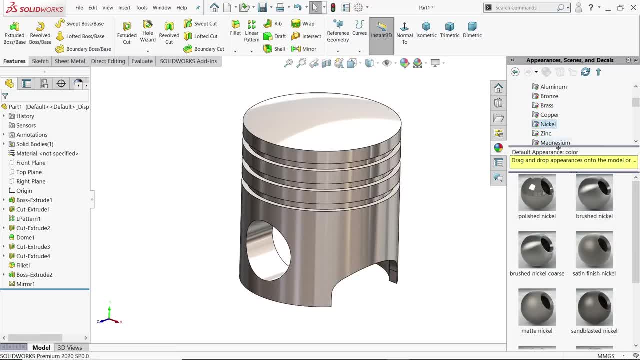 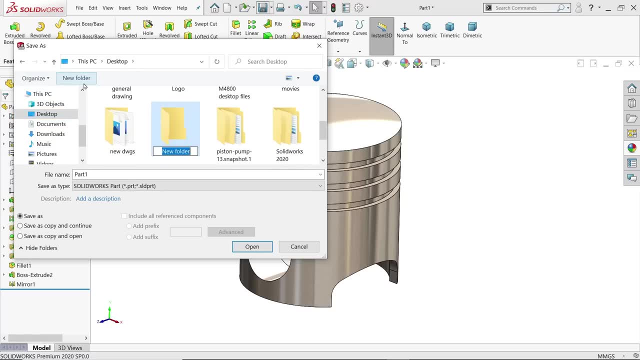 Extrude Boss base. We will choose Nickel Brush- Nickel- Now let's save this one. Go to desktop. Create a folder. Four Cylinder engine, And this is the first part: Piston- Save. Now let's go to new. 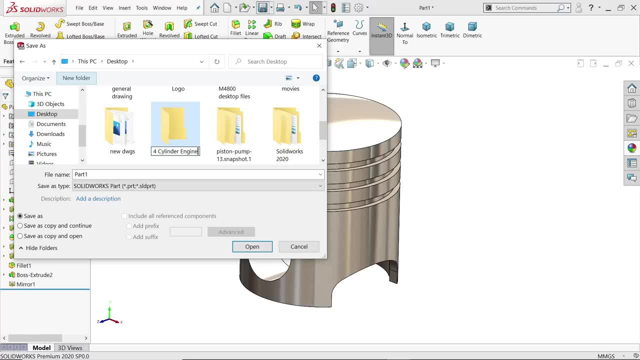 Part: Ok, This is the first part. Piston Save. Now let's go to New Part. Ok, This is the first part. Piston Save. Now let's go to New Part. Ok, Save. 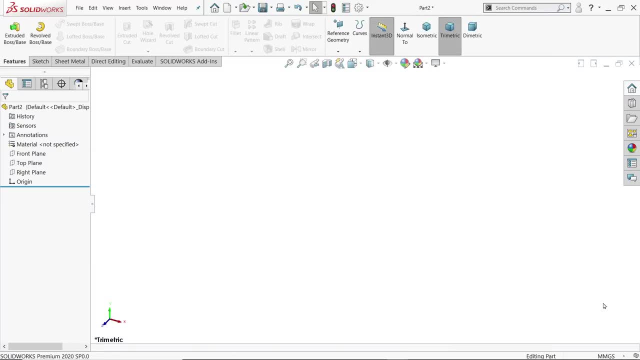 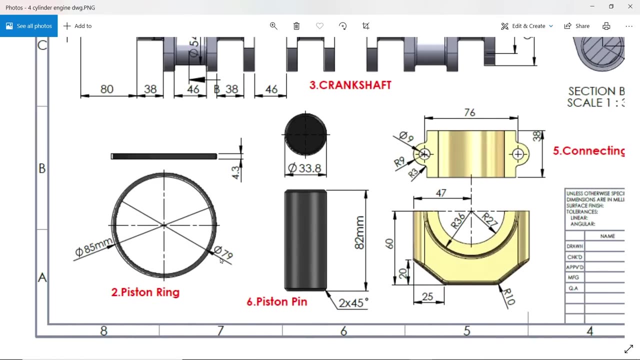 Ok, Unit From You can change it from here. We will keep Millimeter Gram. Second Piston Ring. This is 85 by Internal diameter, 79. 85.. And thickness 43., 4.3.. 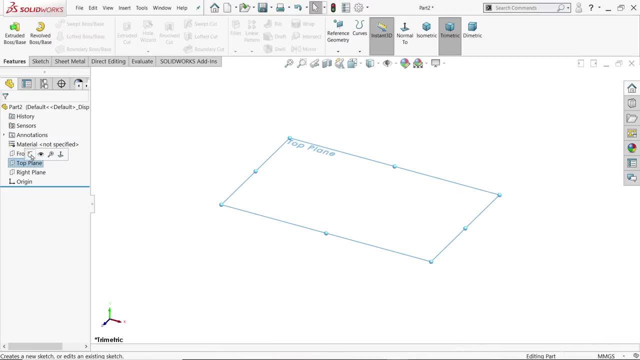 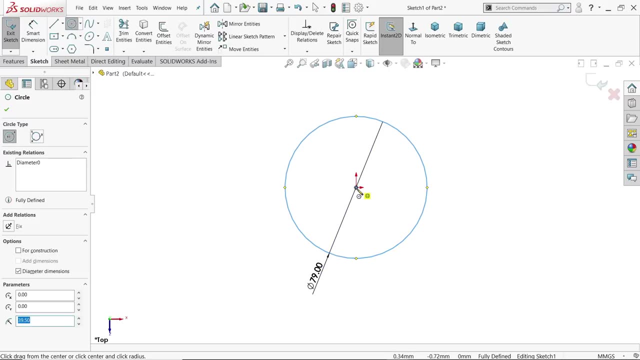 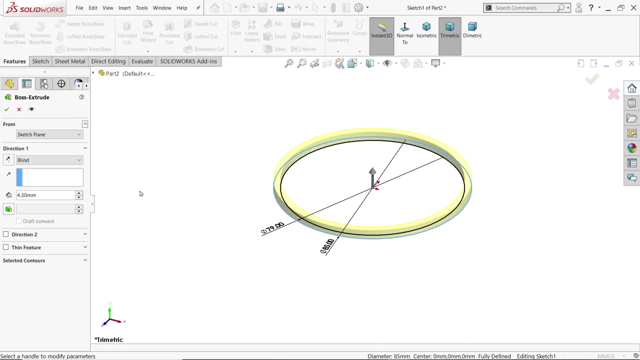 Top Plane Sketch And I will select here Two circles: 79., 85.. And This Is The Top 85.. Go to Feature Select Extruded Boss Base Keep End. 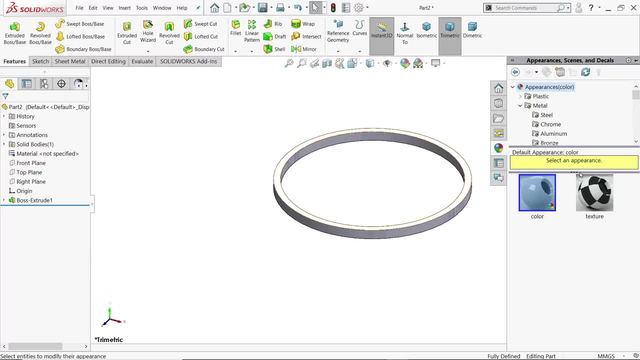 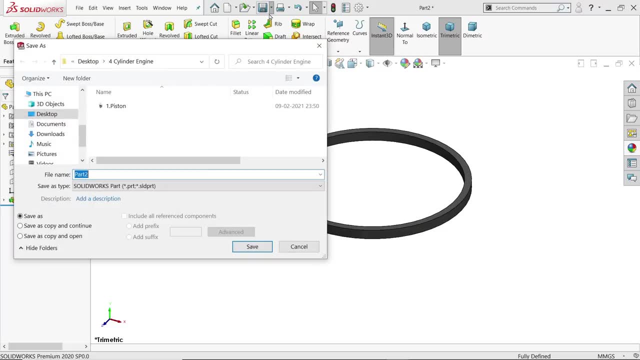 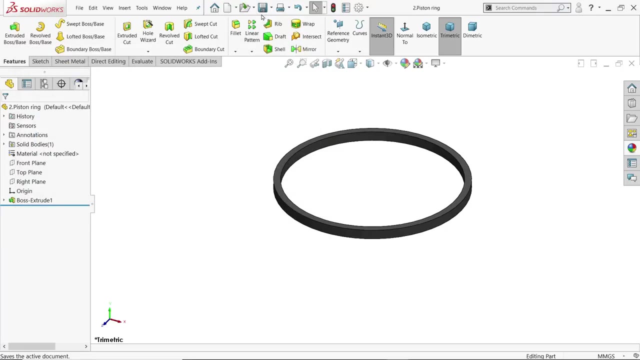 Condition: Blind And 4.3. Millimeter. Say Yes, Ok, Let's Apply Material Rubber. Close The Rubber Now. Let's Save. This Is New. Let's. 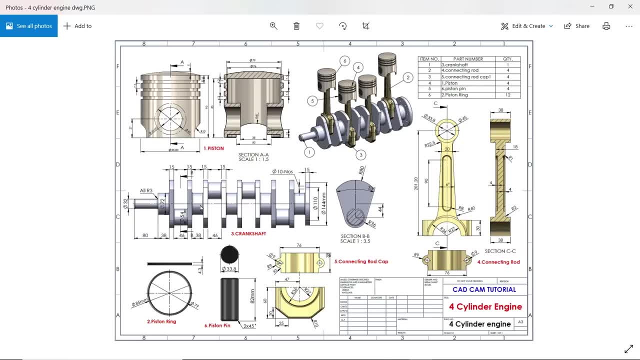 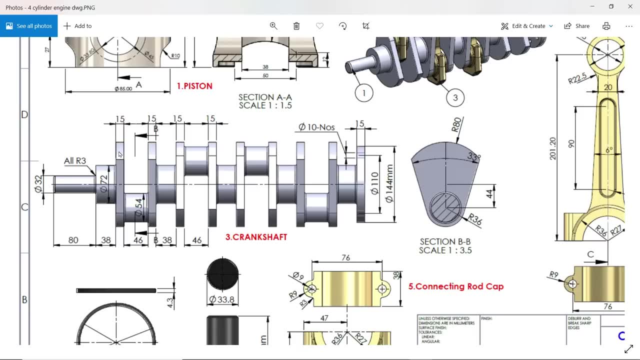 Make The Third Part Here. Third Part Is Very Important Part. It Is Crankshaft. Now, First We Will Start. Half Of The Crankshaft Is 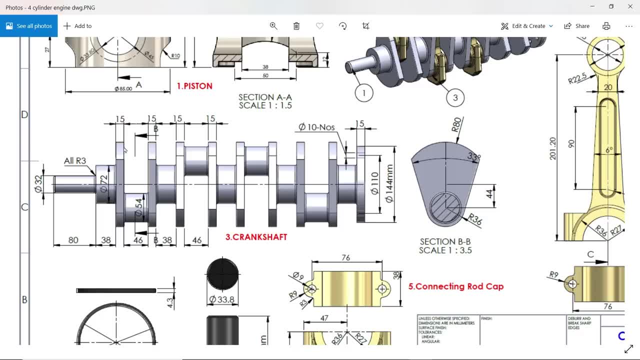 Just Mirror, You See This Thickness Here You Will See Fifteen Millimeter. Then We Will Add This One Forty Six Millimeter Long, Fifty Four. 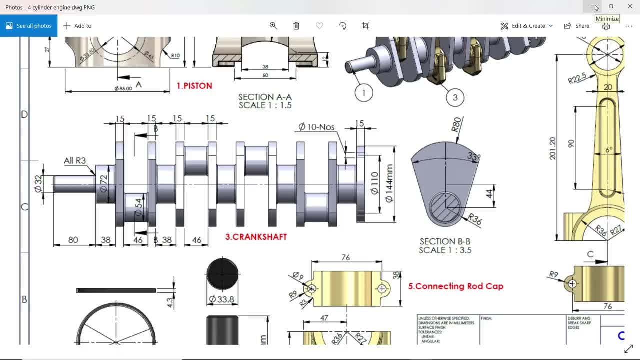 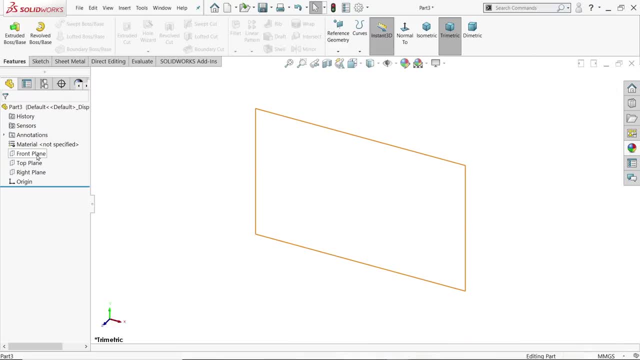 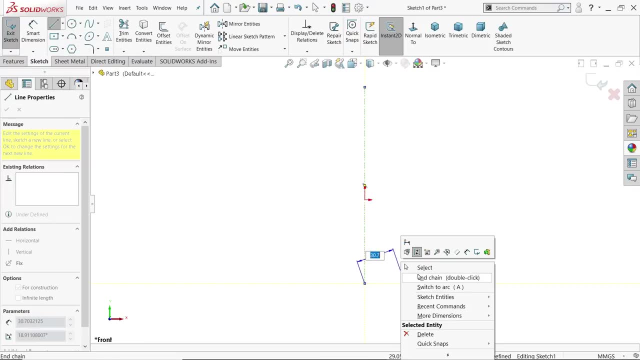 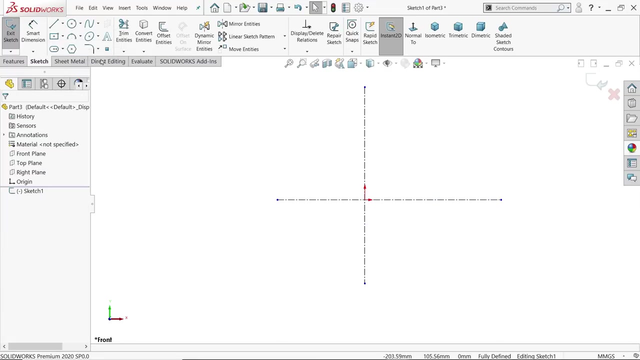 Diameter. Ok, Then Other Side We Will Add. Now Let's Front Plane Sketch. Let Me Draw Centerline. This Is Actually Helpful For Ok, Let's. 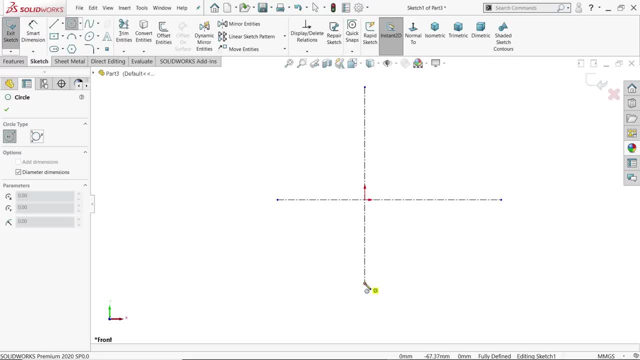 Apply The Bottom One This Diameter Seventy Two. Now Here I'll Select Three: Center Point Arc. This Is The Center. Start From Here To Here. 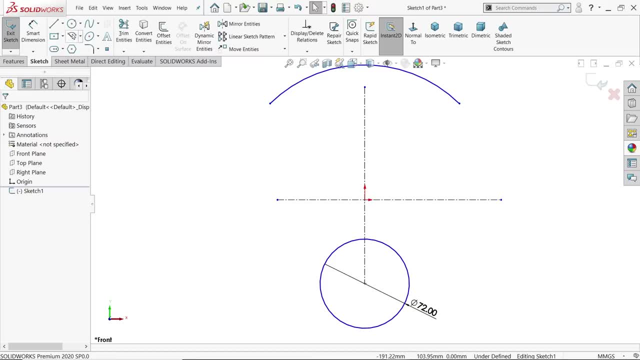 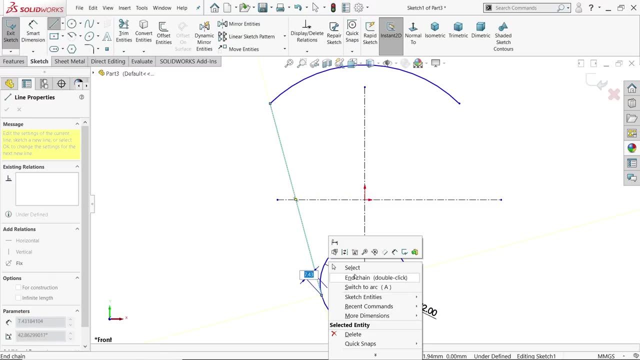 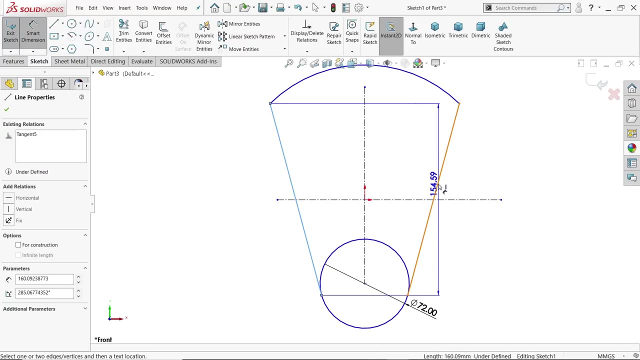 Exit. Now Make One Relation, Hold Both The Point. This Is Tangent Point. Ok, I'll Select This Two Lines That Are Entity It's Mirror. 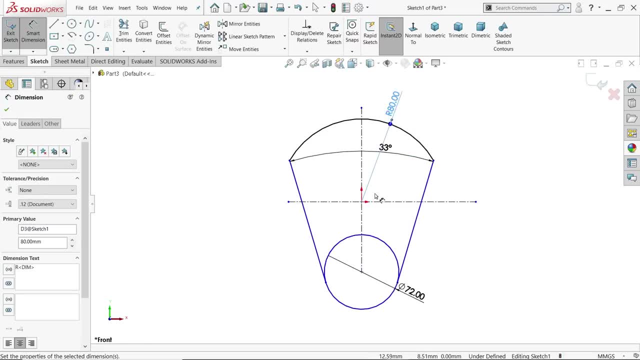 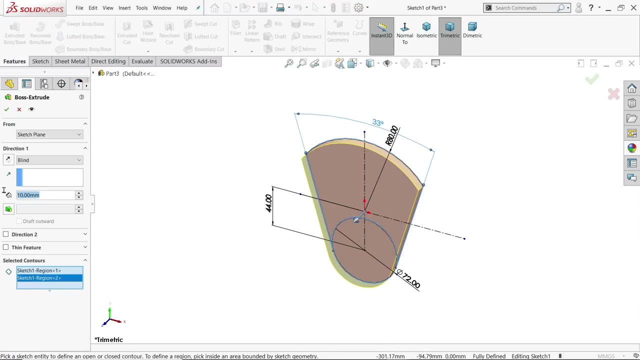 Now Thirty Three Angle, The Radius Eighty Millimeter, See Now Distance From Here To One, One, Two And This Thickness Fifteen Millimeter. Keep And. 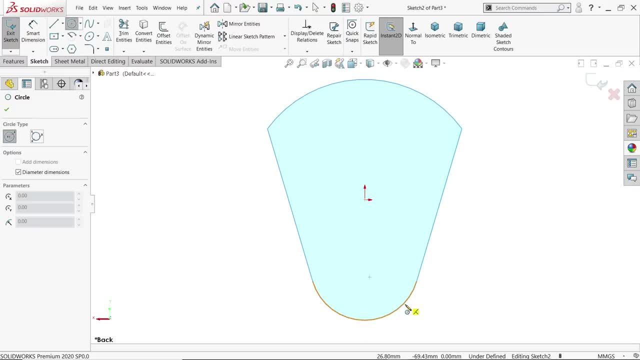 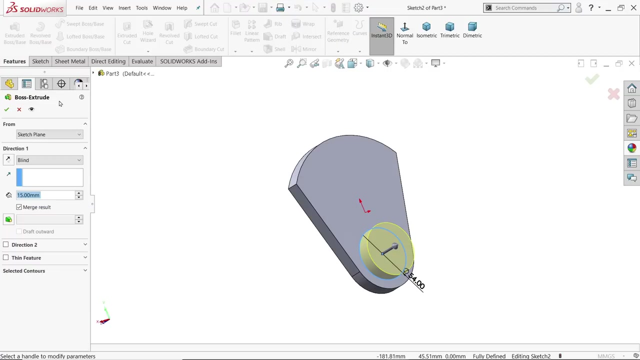 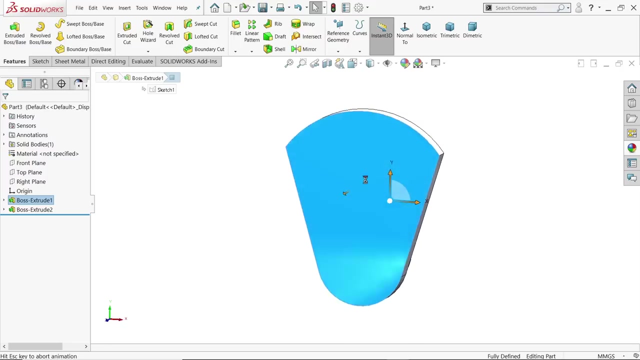 Condition Line: Ok, Select Back Surface Sketch. Now Here We. We Need To Create A Small Circle. Fifty Four And See Here. Ok, Now This Side. 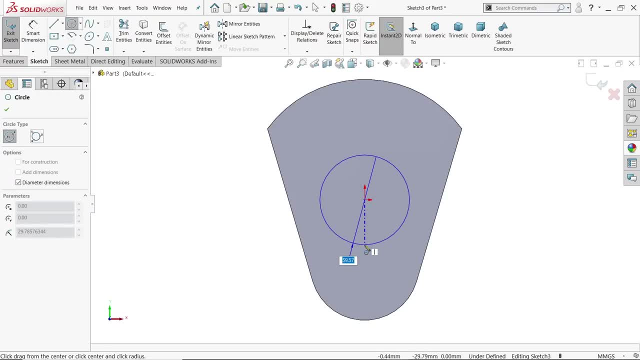 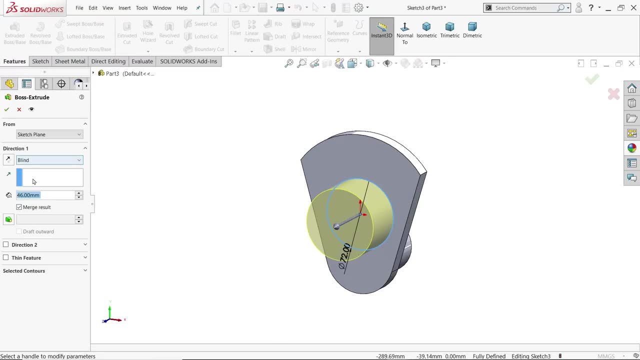 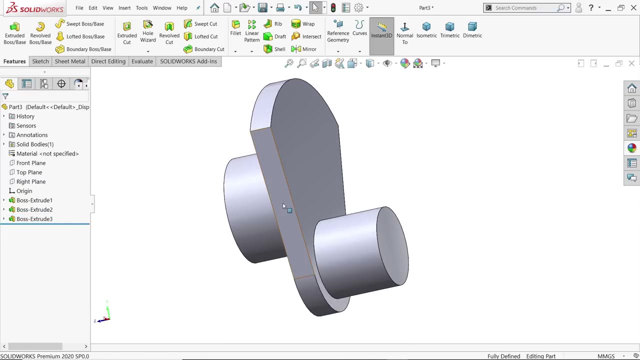 Sketch At Center, We Will Make One Big Seventy Two Millimeter Extrude And This One We Will Extrude Up To Keep And Condition This. 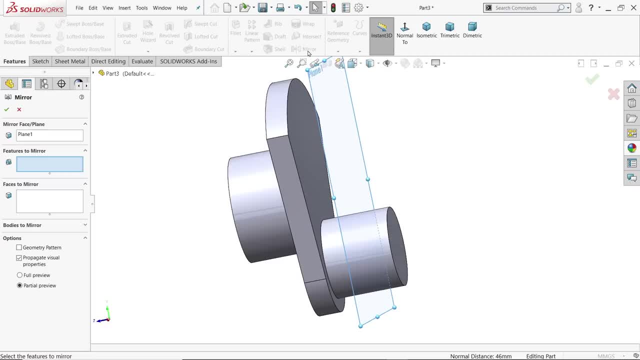 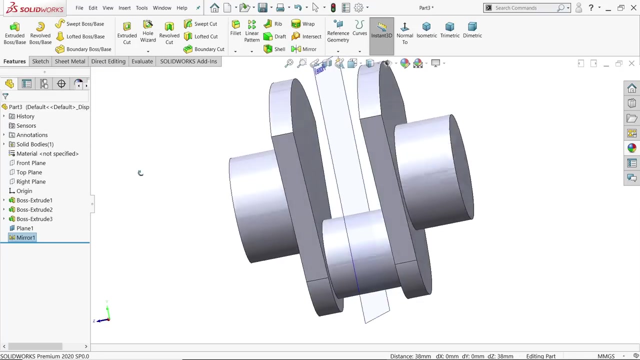 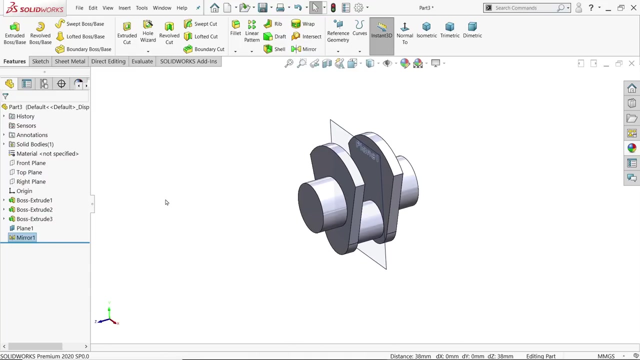 Face. See Mid Plane Going To Create Look Mirror. Plane Is Selected. Now Choose Feature One: Two: Look, Ok, That's It. Now It's Time, But. 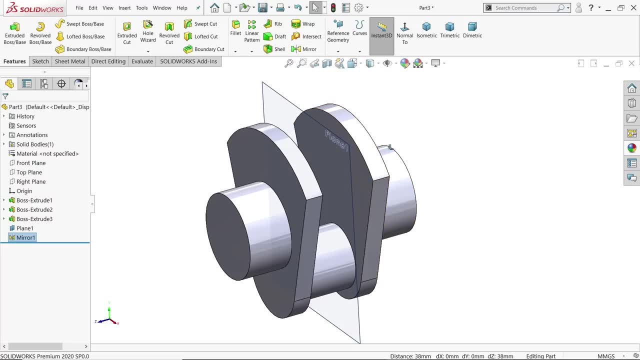 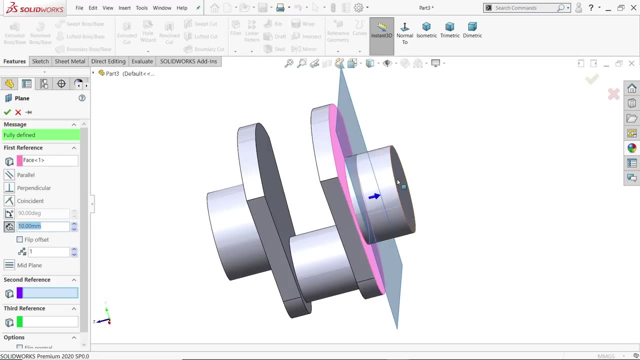 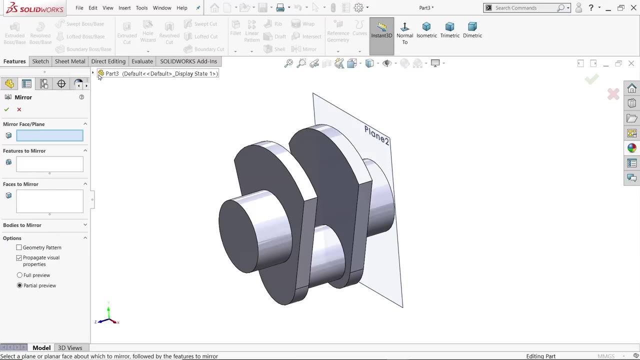 Reverse. So We Will Do One More Thing, Just Hide This One Again. Create A Plane Between These Two. See, Let's Try To Make Mirror. 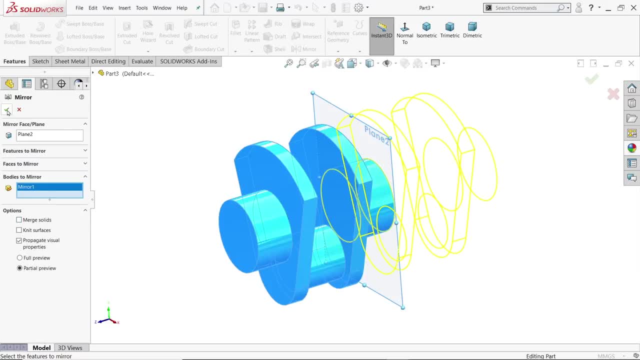 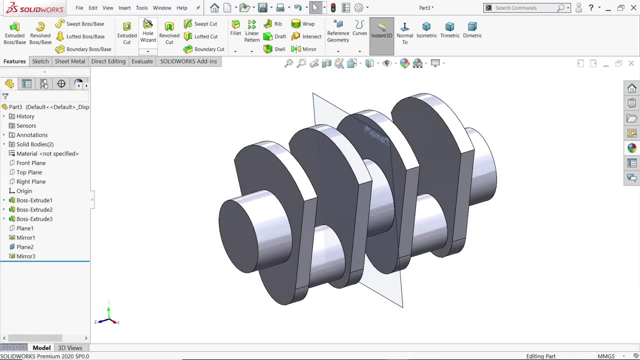 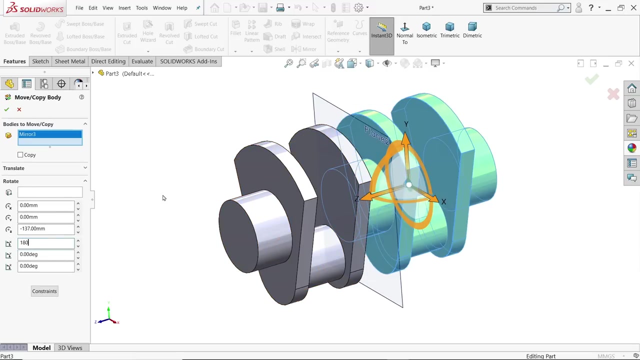 Now This Is Body. Ok, So Now, Here You Will See Two Bodies. Now We Want To Rotate, So Just Go To Insert Features And Here 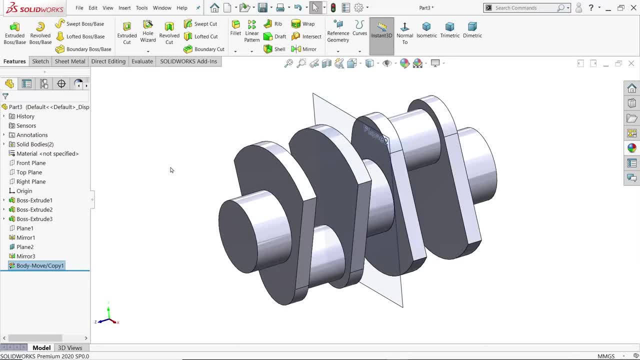 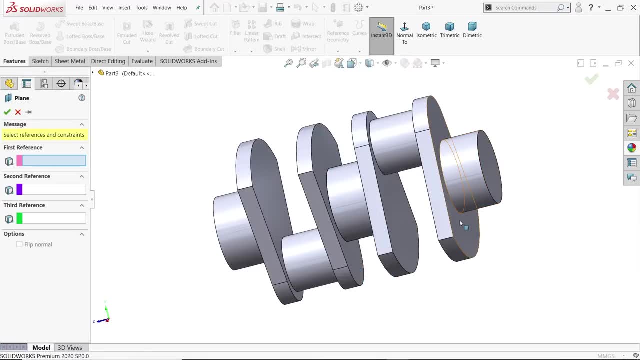 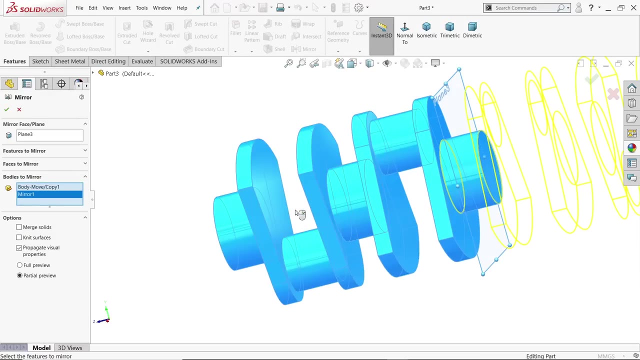 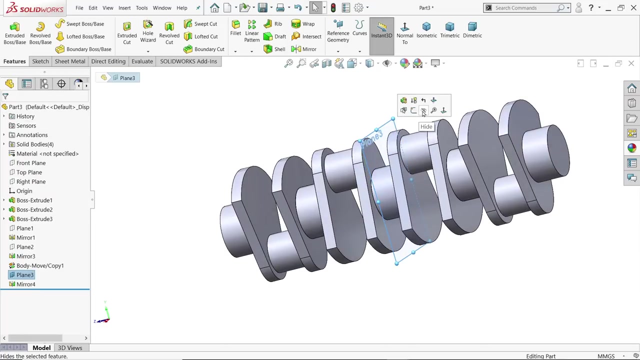 You Will Find Option Move, Copy, Select, Hide Again, I Will Create A Plane In Between These Two. Ok Mirror. Now, Here I Am Going To. 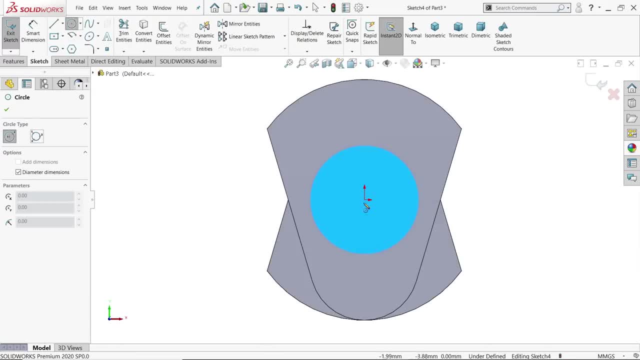 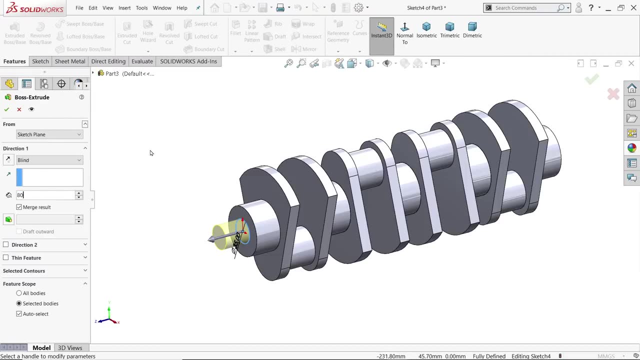 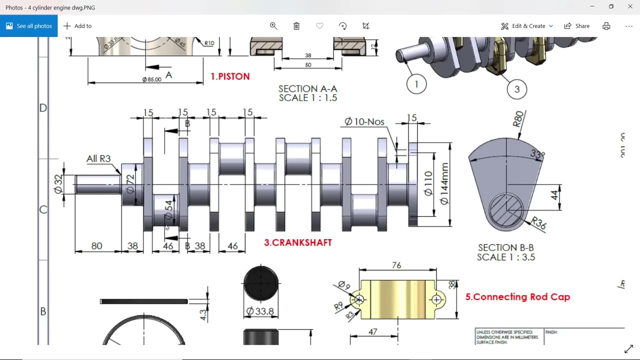 Mirror These Two Bodies. Ok, Look, Let's Hide Sketch 35.. Extrude: Ok, Now See, This Is The Things. Everything Like 15mm Thick, Everything. 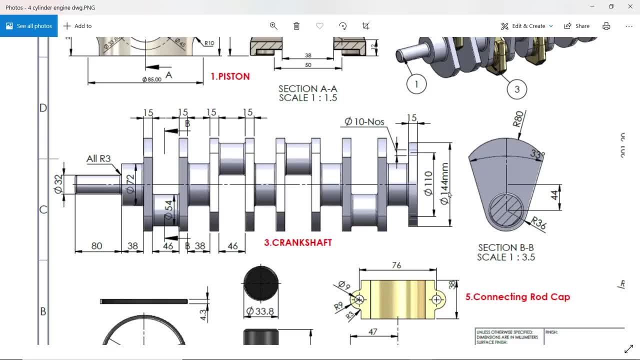 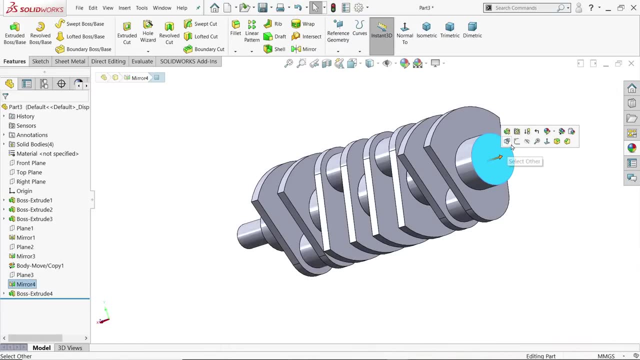 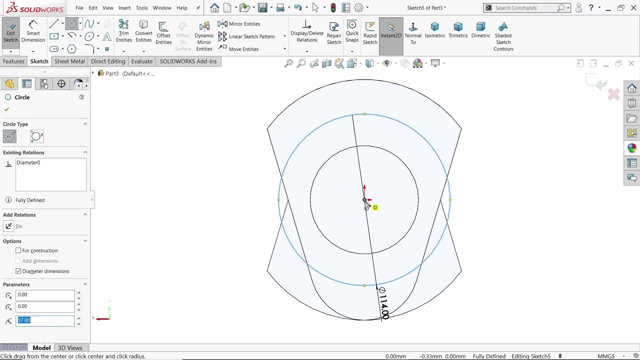 We Did Perfectly Radius 3mm. Then There Is Outside, This Is One Circle 144mm, And There Is Sketch And Here 114mm Again. 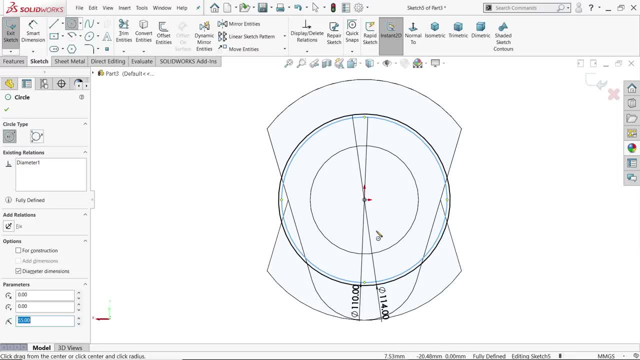 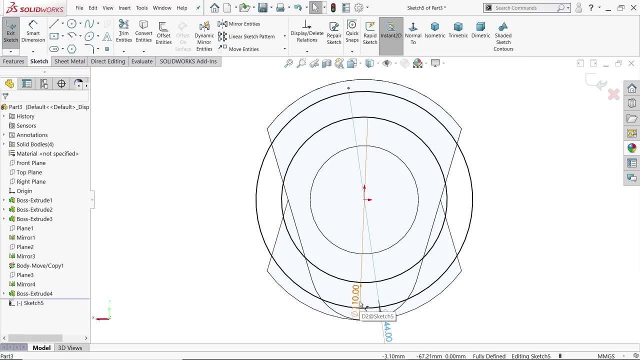 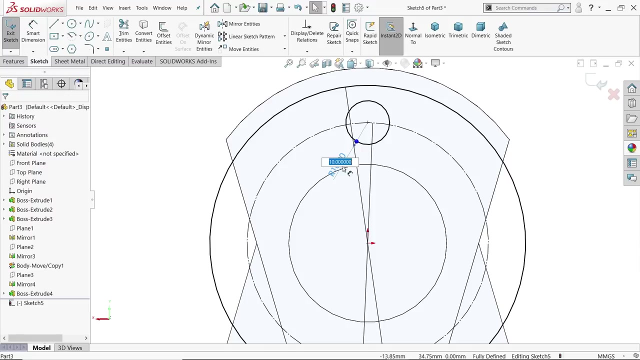 One Pitch Is 110mm, This Is 144mm. This Circle Make For Construction Again. Small Circle Here Is 10.. Not Radius Is Diameter, 10.. 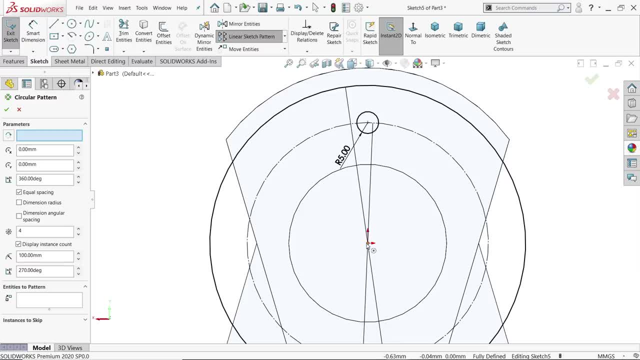 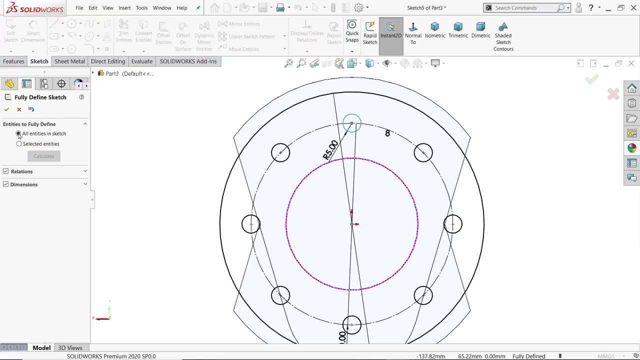 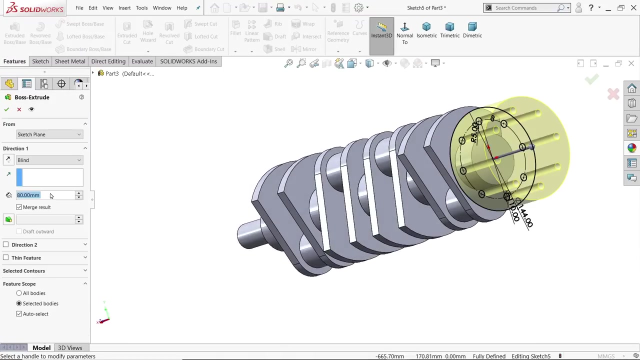 So 5. Radius Circular Pattern: Center Point Here Select The Circle And Make Number Of Patterns. 8. Say Yes, Now Go To Extrude 15mm. 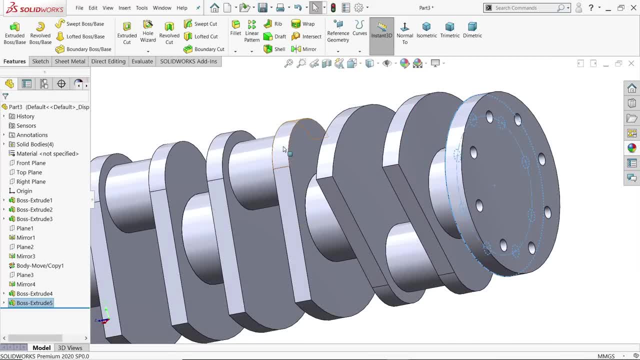 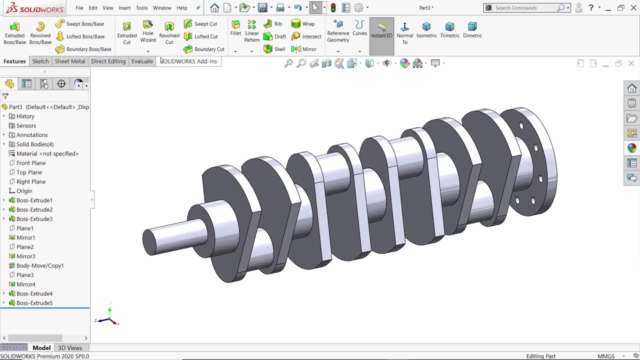 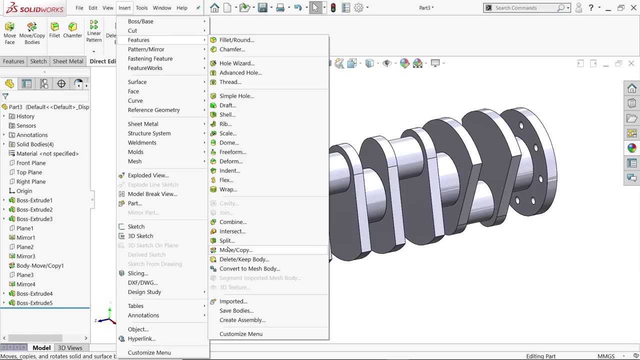 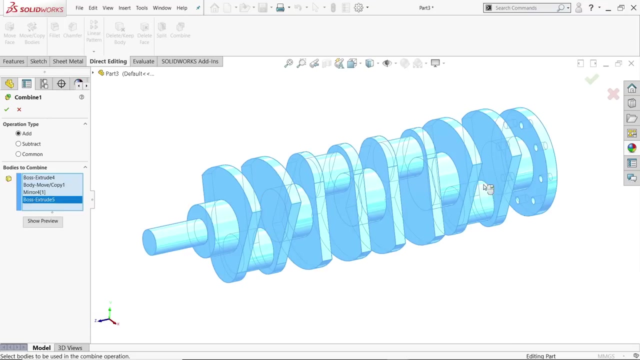 Is The Thickness. Look Now, Let's Combine All Body Direct Editing. Here You'll Find Option: Combine Or Even Though Insert Feature, Add Here. Okay, Now. 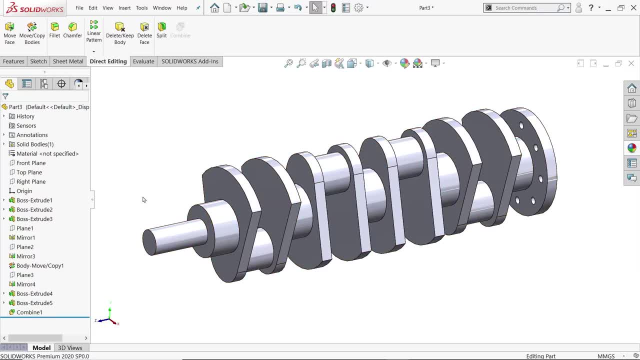 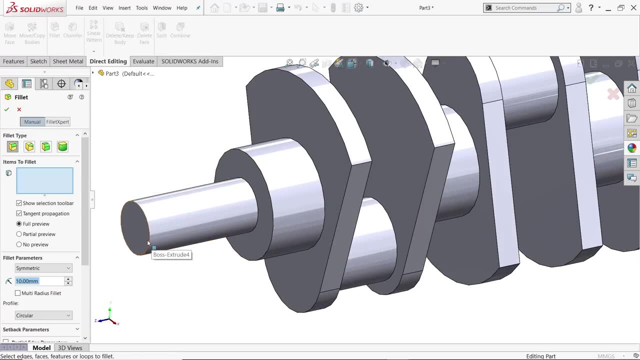 Here Only One Body. I'll Select Fillet. I'll Choose 3mm One. I'll Select This One, And Here I'll Find Option Like This: 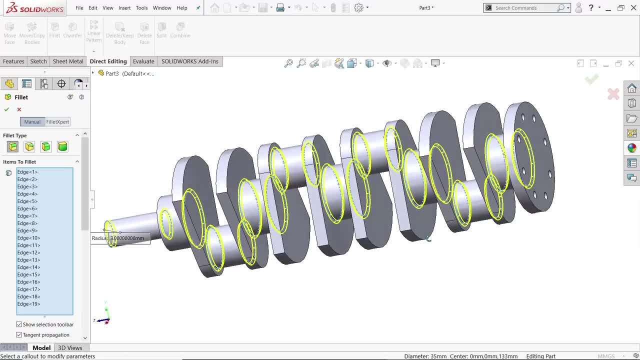 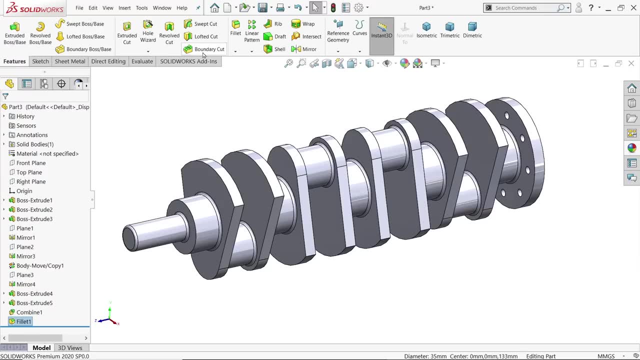 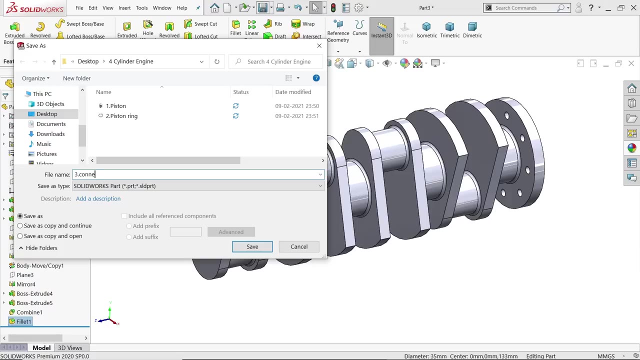 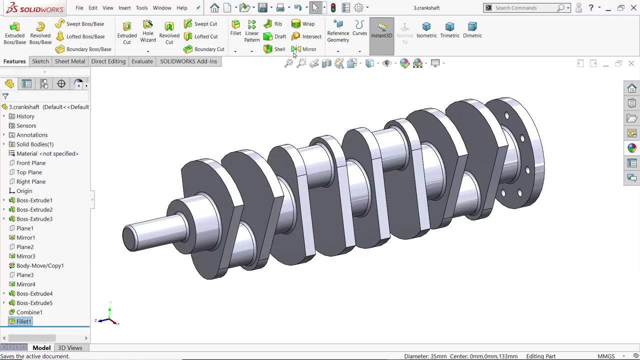 If I'm Going To One Body Editing, You'll See No Need To Choose One By One. This Is The Part Number Three Connecting Rod Oh. 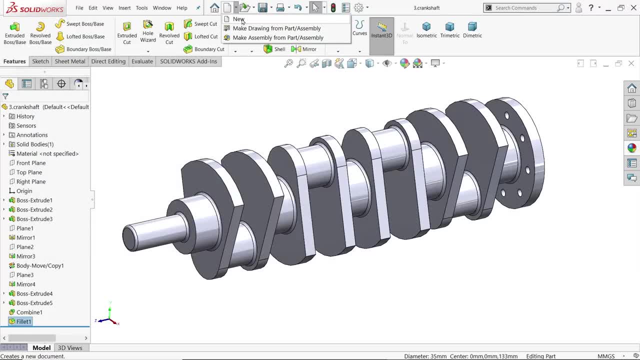 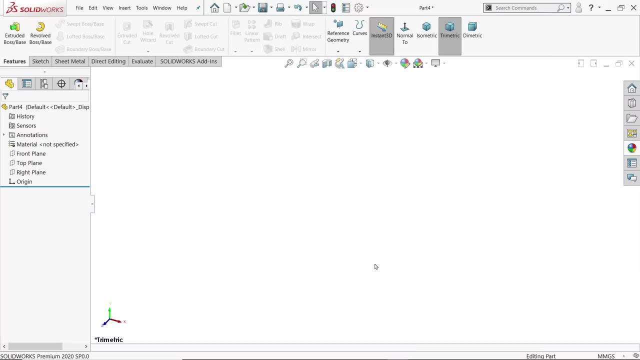 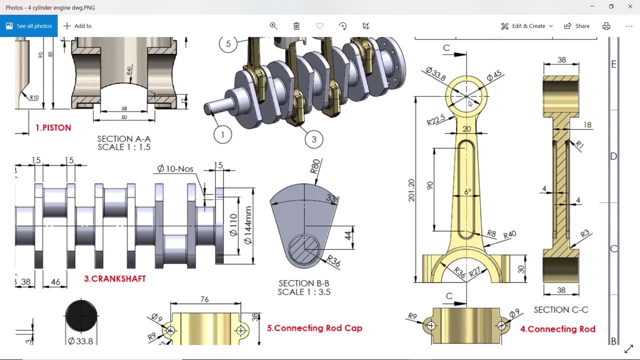 Sorry, Crankshaft, Let's Do A New Part Now Here. The Next Part Is Connecting Rod. This Is A Very Important Part. The Length Of 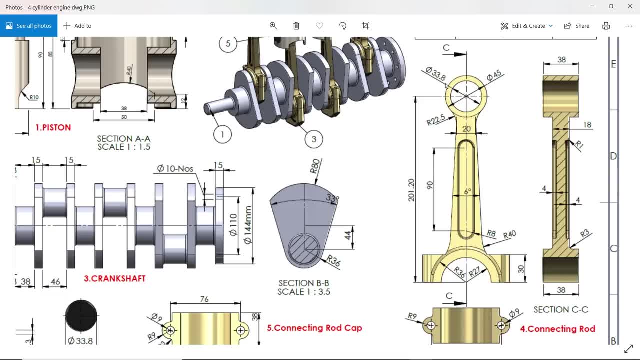 Connecting Rod. Two Hundred One Point Two. This 33. And 45. This One Extrude 38. Millimeter. Okay, Then This Middle One, It's 20.. 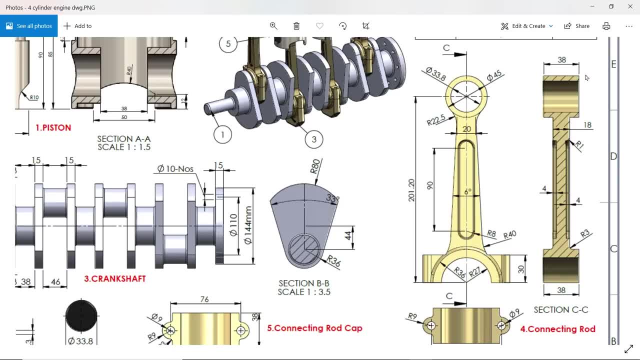 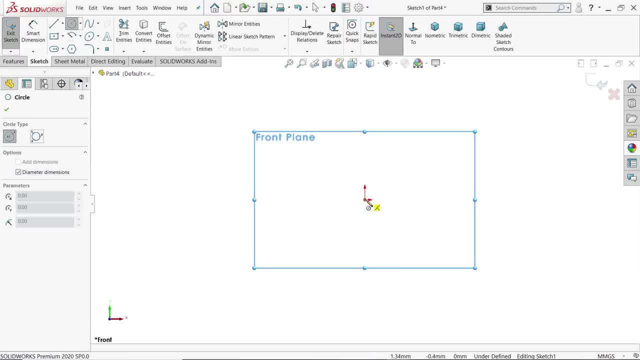 This Is The Distance And Angle Six, And This One We Need To Extrude 18.. Millimeter: Let's Make This Basic 33. Point Eight: 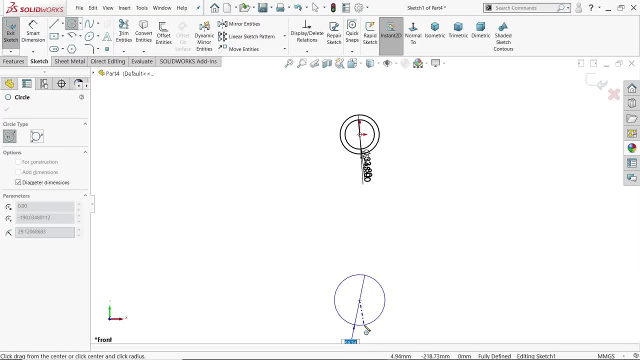 Now Here The Bottom One: 30., 27. Radius Into Two. Now The Another One Is 36. Into Two. This Is Let's Connect With Centerline. 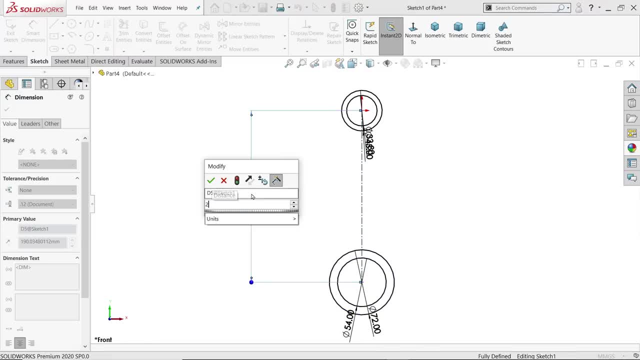 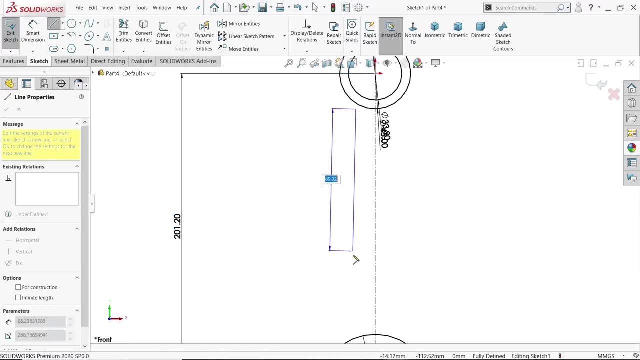 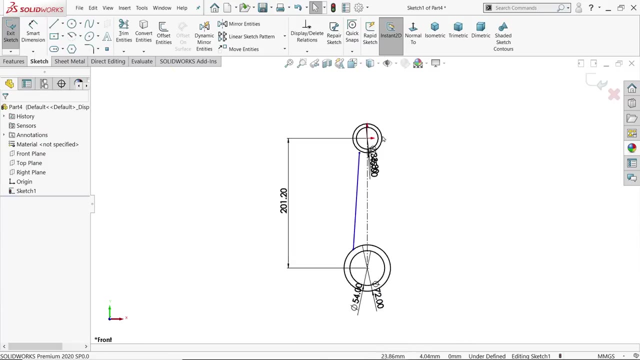 Make Sure 201.. Point Two: I'll Select Here Line And I'll Connect From Here To Here. I'll Select Okay, Let's Connect It First. 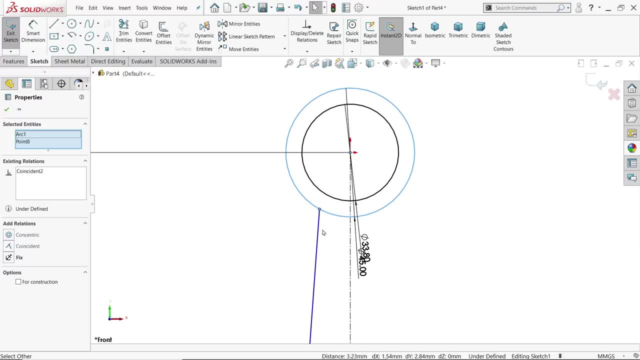 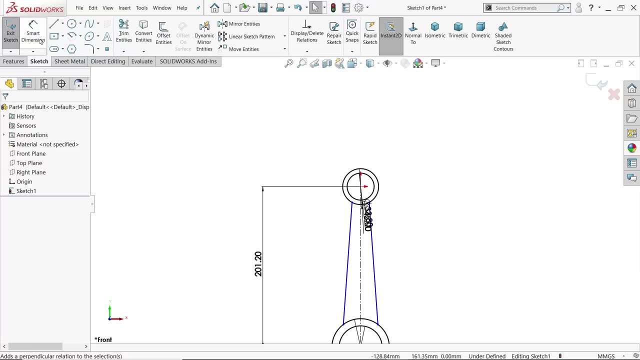 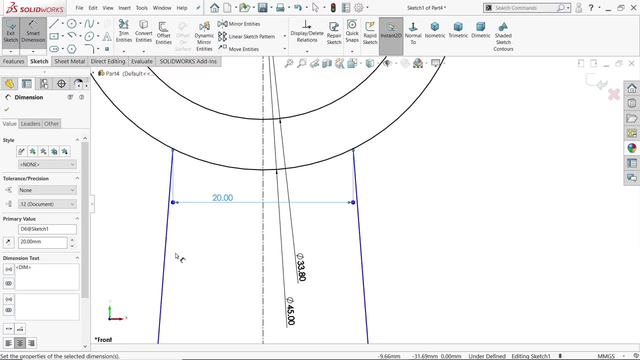 Go Inside If I'm Going To Select Directly Mirror. Now, This Distance, It's 20. And The Angle Is 6.. That's It, Extrude. 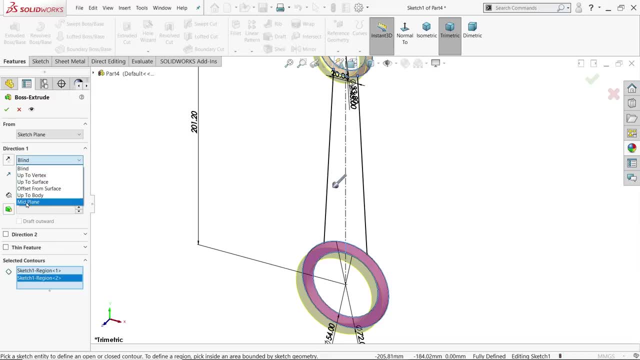 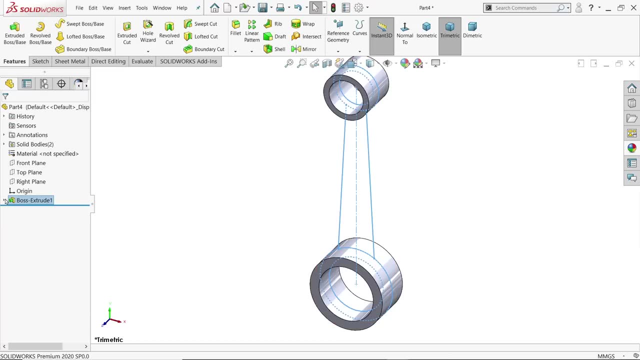 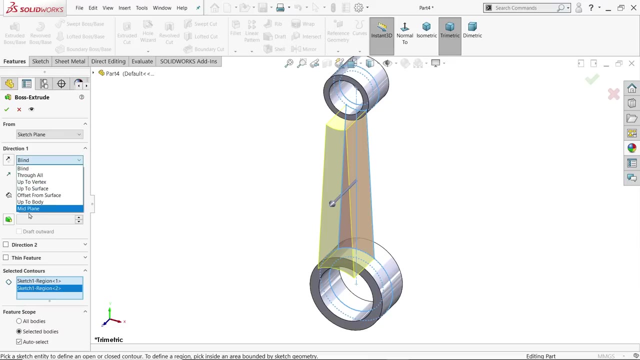 First, I'll Choose This One, This One. Keep Extruded Dimension. Say Yes Again. Select Same Sketch. Extrude This Time. Choose This Middle One Same. 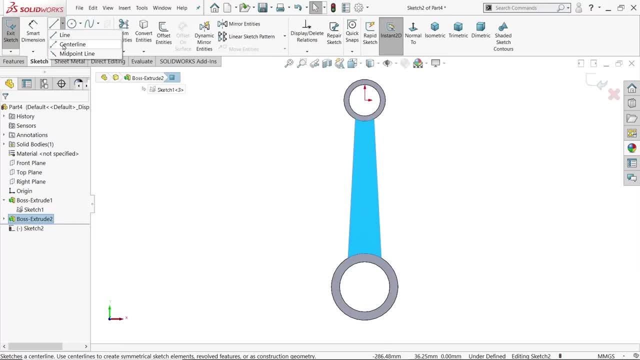 Condition: Mid Plane: 18. Millimetre Center Distance: Okay, If There Is One. What Is Now This? Length: 90. 8. Millimetre: Okay Now. 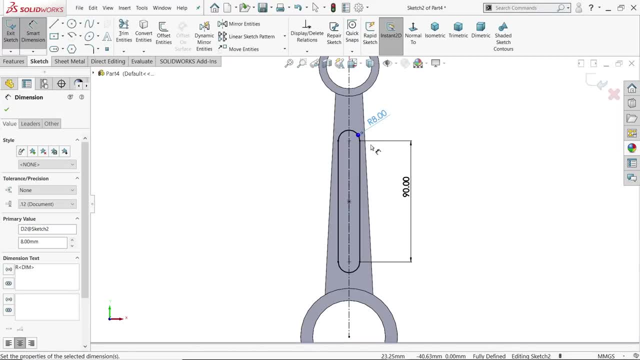 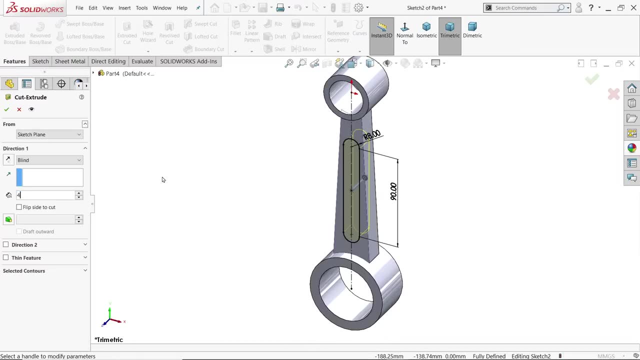 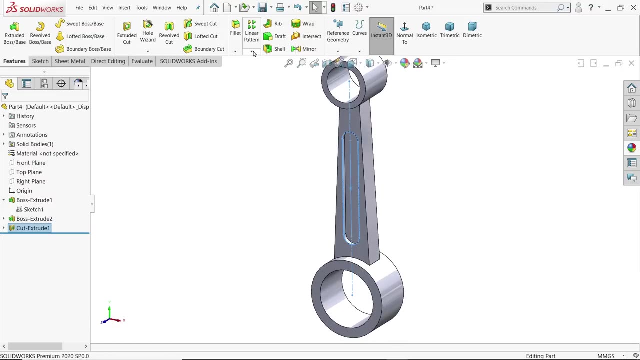 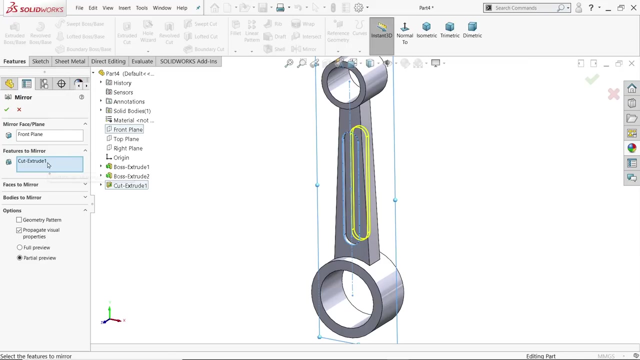 This One We Need To Cut And The Depth Is 4. Millimetre. Let's Mirror Against Front Plane. Okay, Fillet I'm Going To Choose. 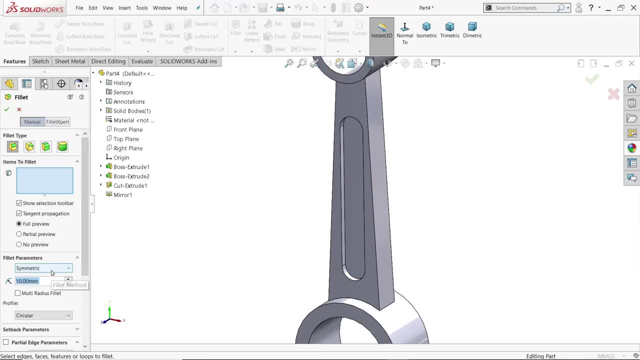 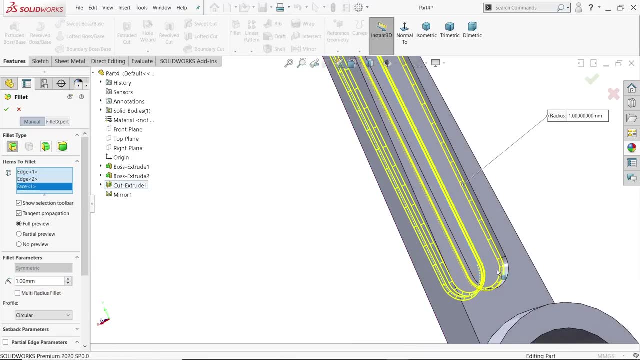 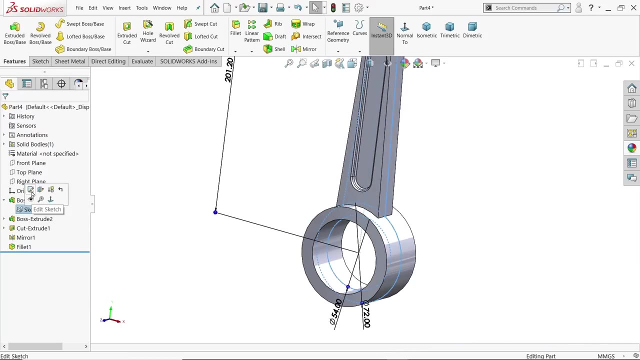 Fillet One Millimetre And I'll Choose This Age Face And This Age. Now Here One Catch In The First Drawing. I'll Select Line. 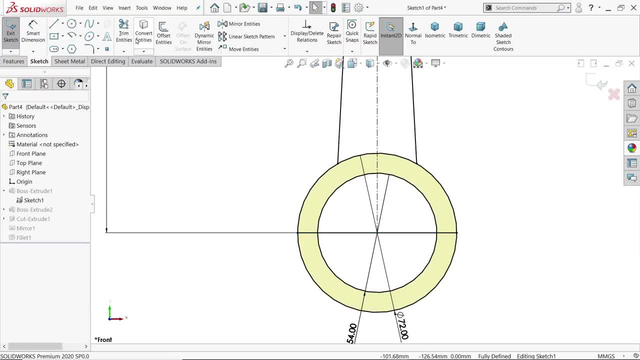 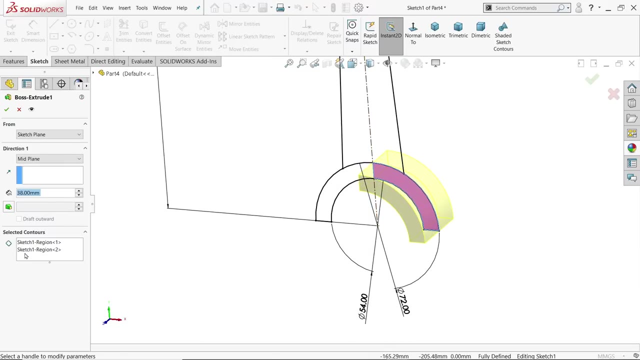 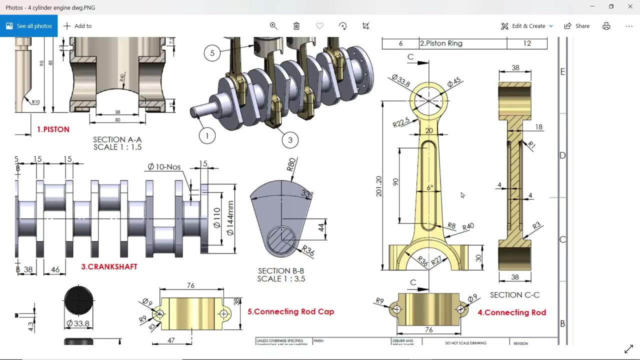 It Should Be Half Trim, Entity Trim. Okay, See, We Don't Need This. Exit Now. Edit Now: Here In This Is Sketch: Select This Also. 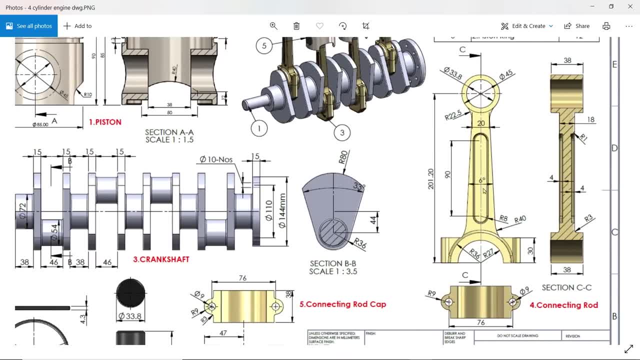 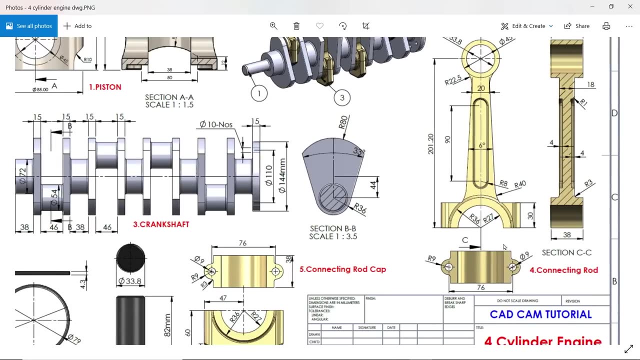 Okay, Look, If You Have This, Edgar, Look At The End Of This. All The Platform, This Area. Okay, At The End Of The System, This: 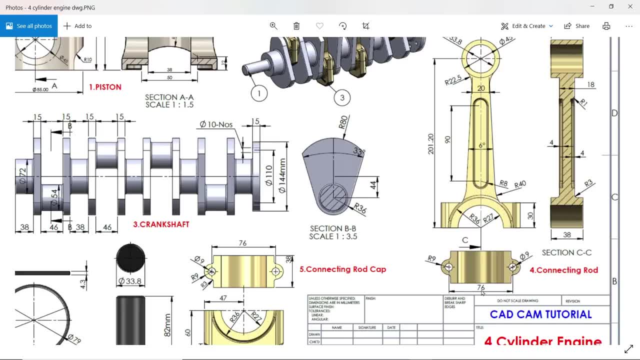 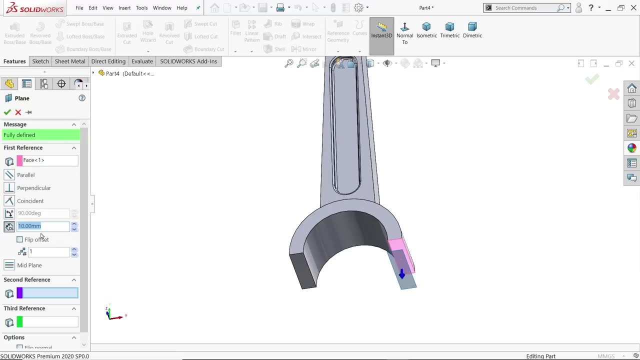 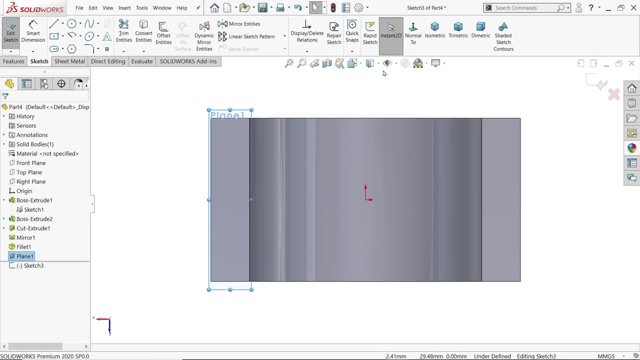 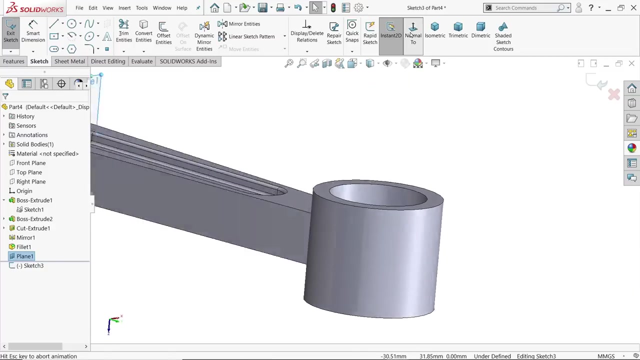 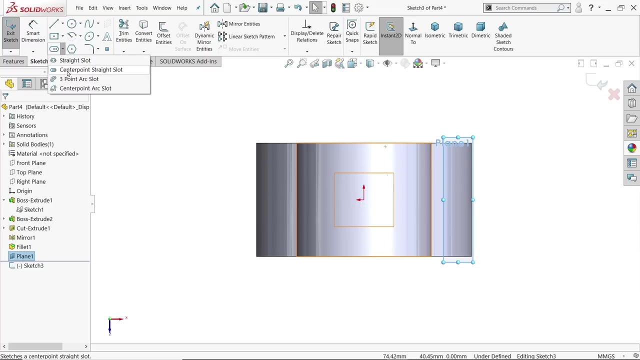 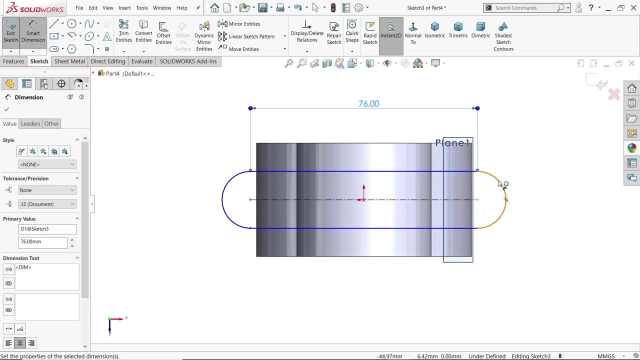 Is One Dot Line. 6th Distance Plane: select this 30, click flip so it moves upside. ok, Sketch Reverse: ok, I will select here Center Point, Arc Straight Slot Distance: 76, 9 Radius. 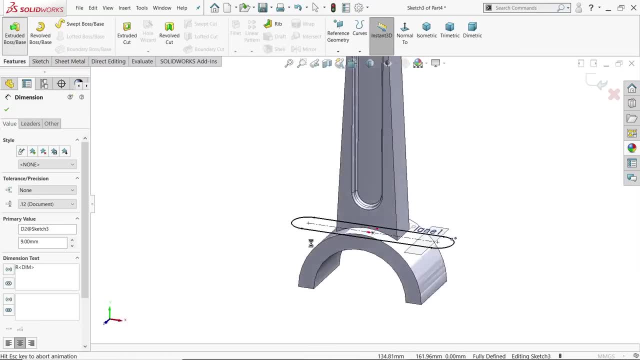 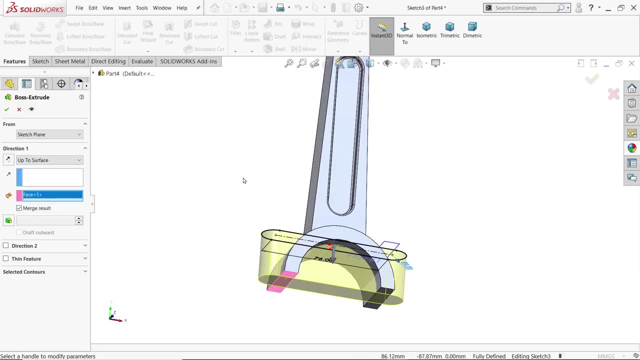 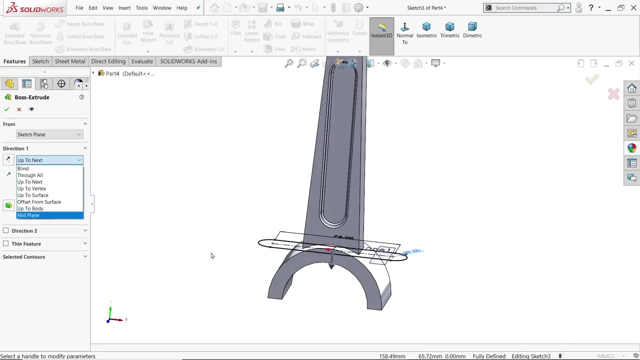 Extrude and we need to extrude up to surface. I will choose surface and I will choose this surface. or let's try up to next. ok, next is not the suitable thing, even up to body. also not suitable thing. up to surface is sorry. 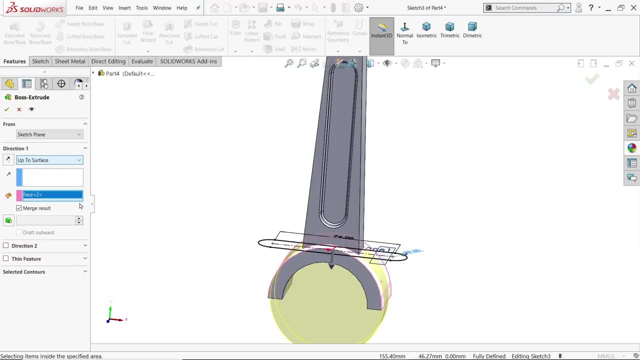 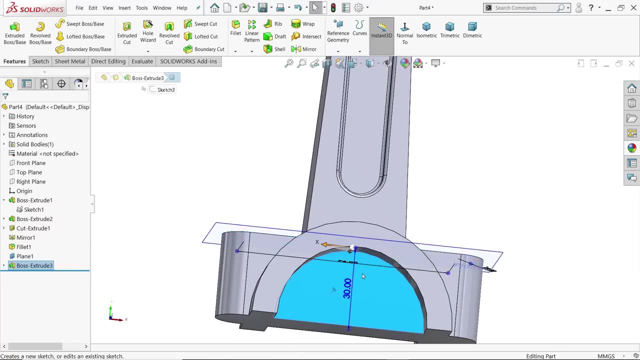 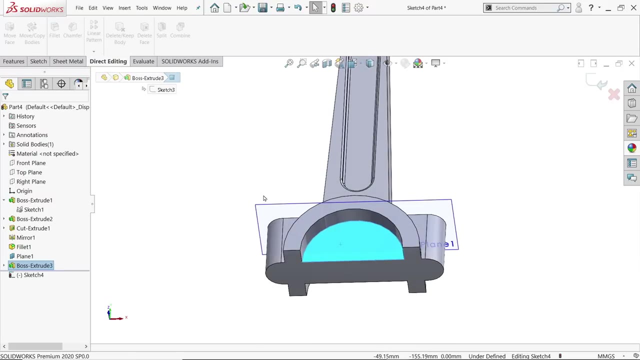 up to surface clear and surface bottom one. ok, Sketch. now we need to trim this one. either there is one option you can directly delete, or something like this, or you can simply use Convert Entity Feature Extruded Cut. keep your end condition through all. 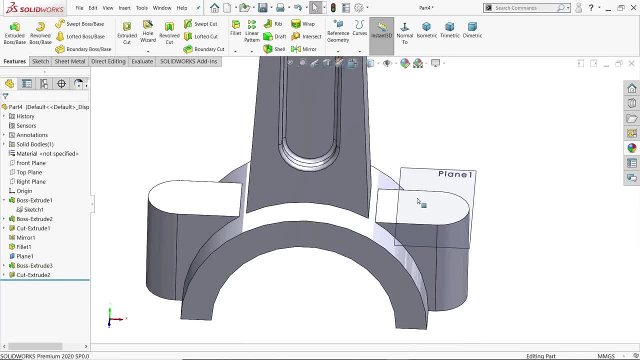 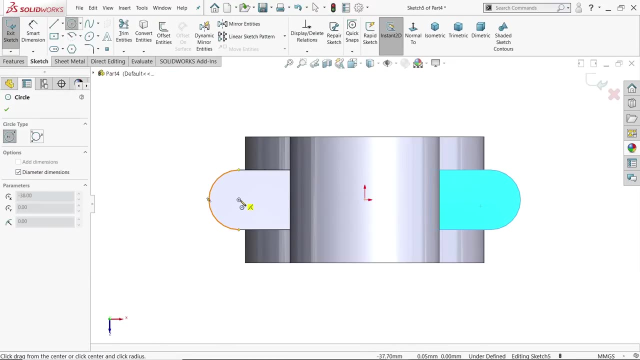 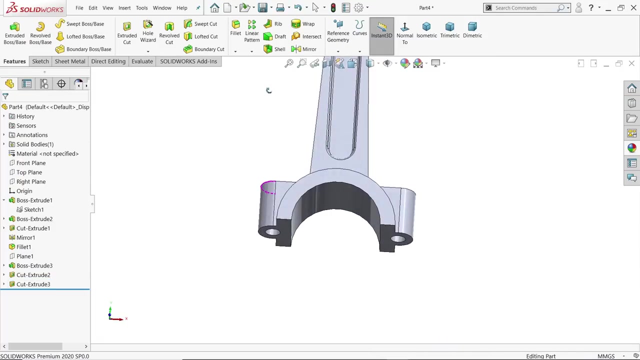 yes, That's it: hide Sketch. now here we need to make hole, and that is 9 mm Extruded Cut and keep end condition through. all That's it. But before going to do this, we need to create Fillet just upside Fillet 40, I will select. 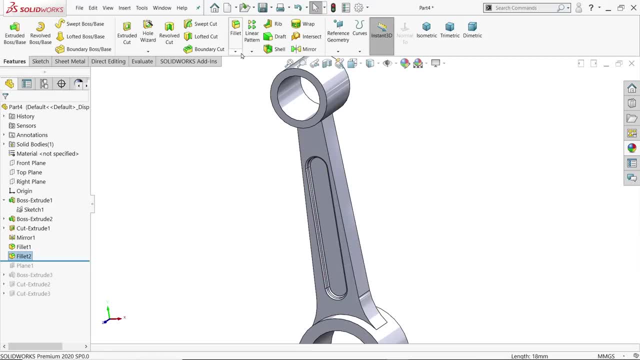 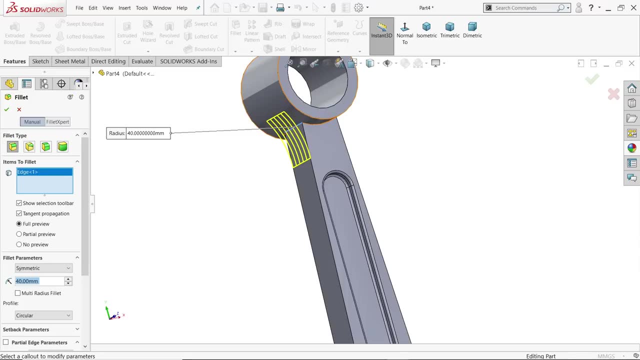 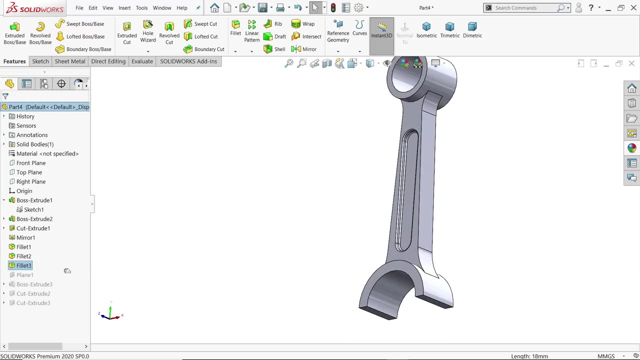 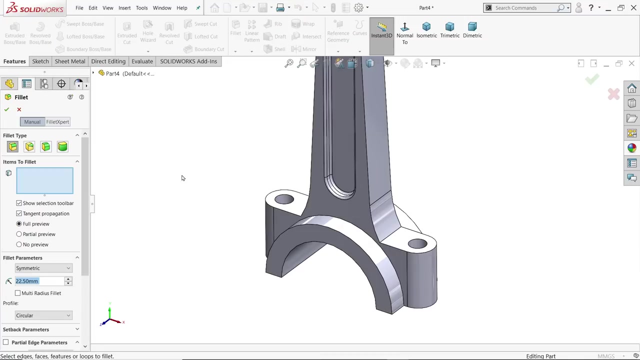 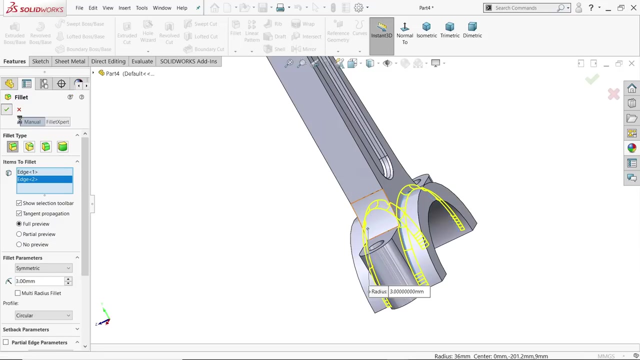 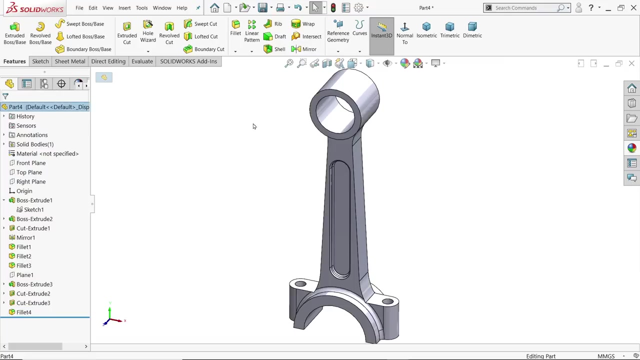 these two edges: ok. Again Fillet: Ok, 22.5,. ok, now comes down. look how this is looks: 3 mm. I will select one and this edge For material. we can give any material, but for proper visibility I will give this metal. 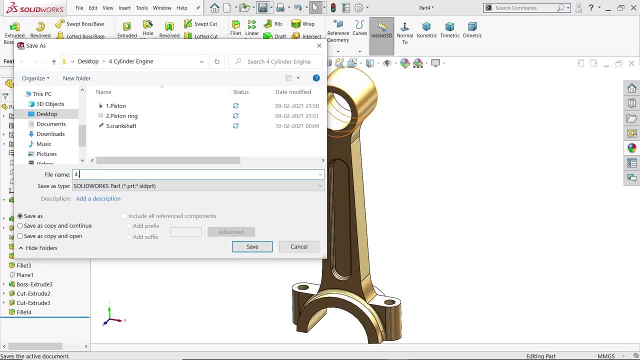 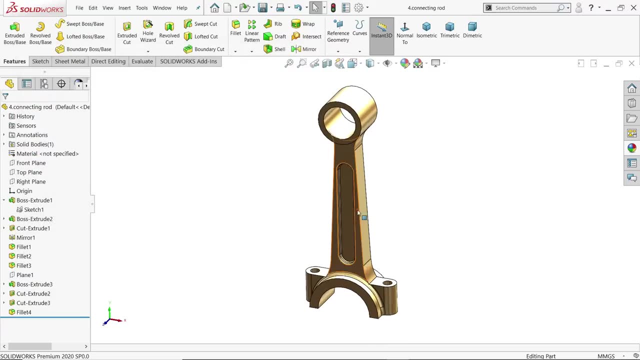 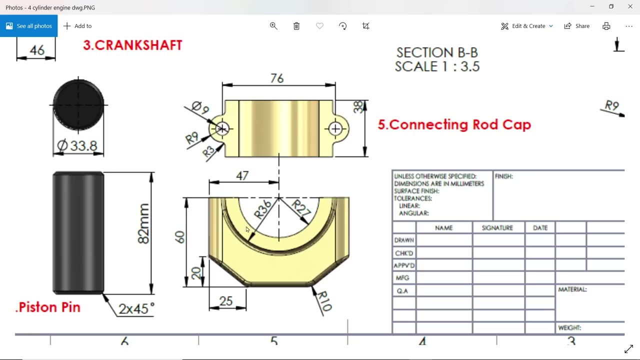 Gold Connecting Rod. Let's make Connecting Rod Cap The same diameter, 27 inside 37 outer one, and this one we need to extrude here, see 38 mm. Then we need to make this external body 60 mm away from here. this cut out 20 by 25,. 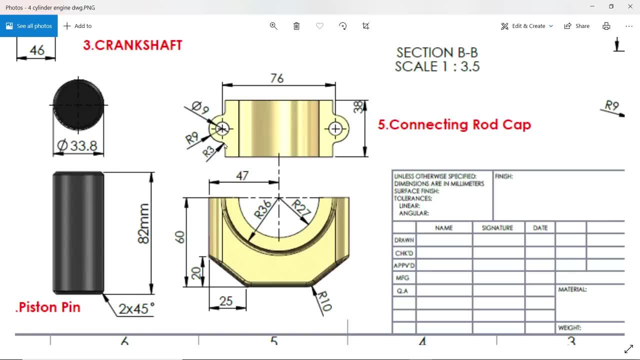 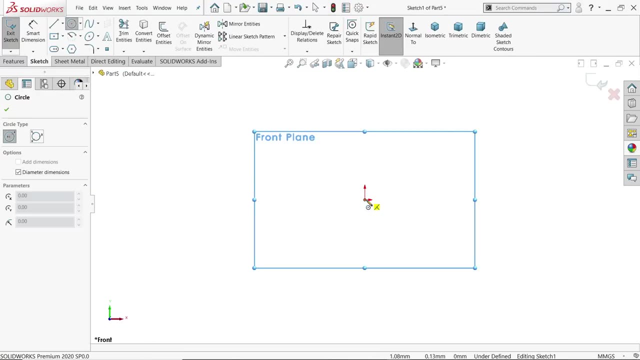 corner radius R10.. And here also this corner radius R3.. And the same, this cut R9, outer inner diameter 9,, 76 mm. ok, 27 means 54,, 72,. it's 37, line. 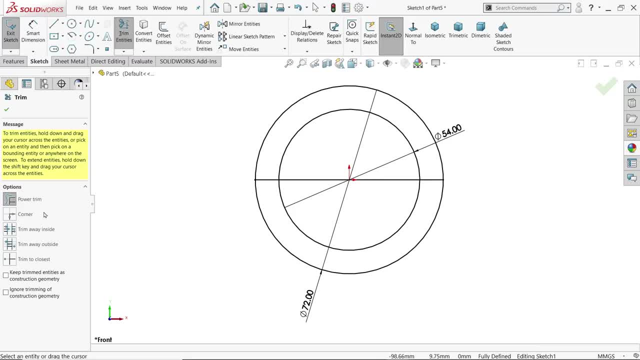 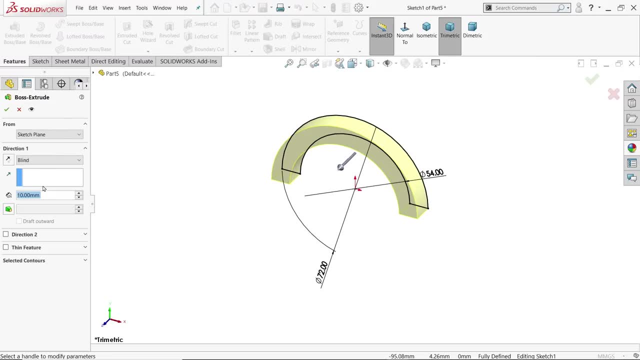 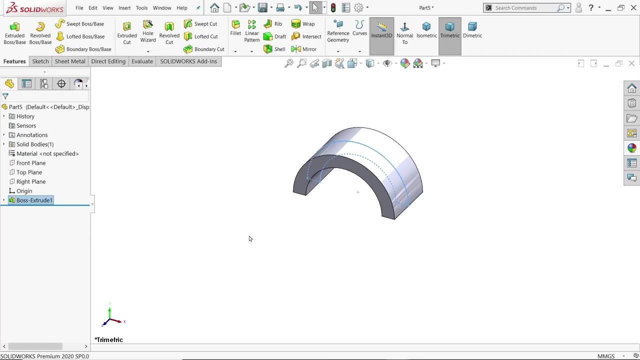 Connect Trim Entities, Power Trim, just Trim, we don't need this. lines Extrude 38 mm. keep end condition: mid plane. look, this is perfectly, is defined. now let's make one plane 60 mm. 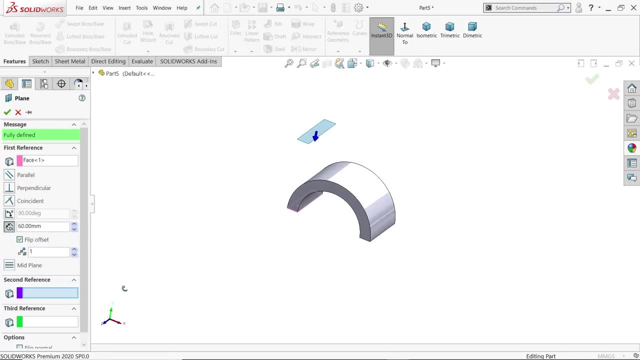 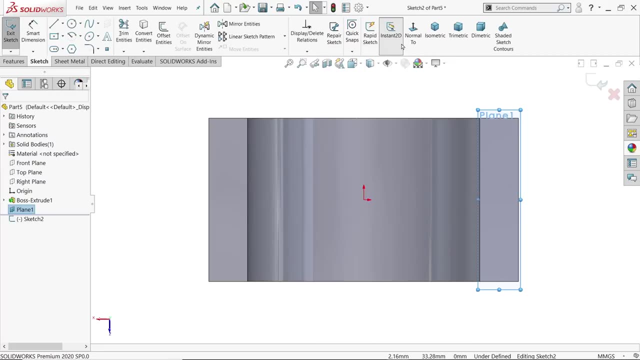 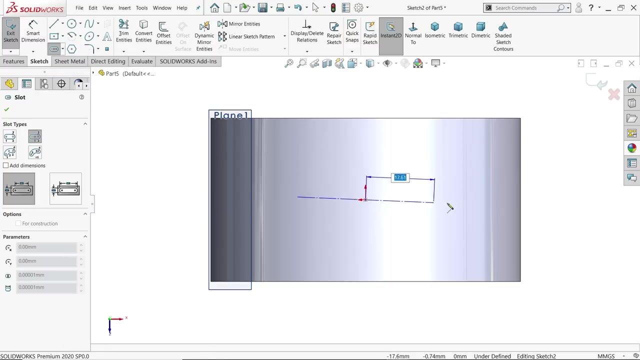 60 mm flipped side ok sketch. I'll again reverse and center point straight slot the length 76, radius 9 mm. 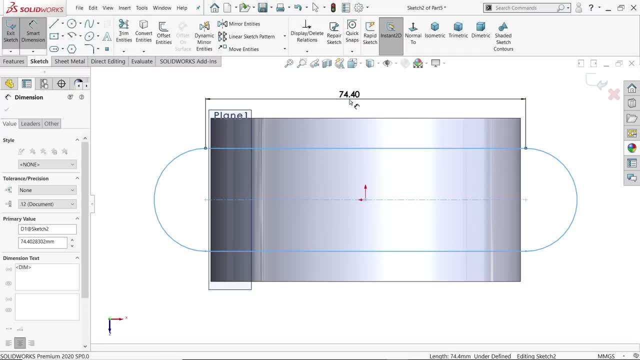 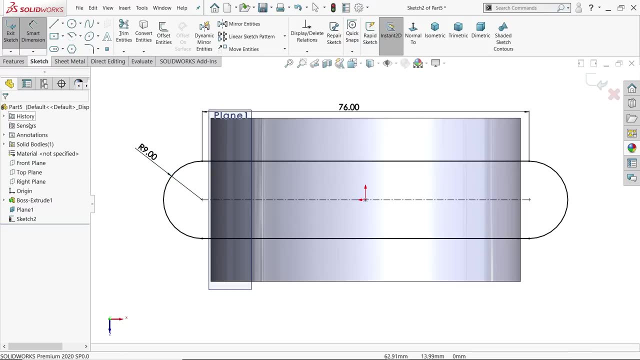 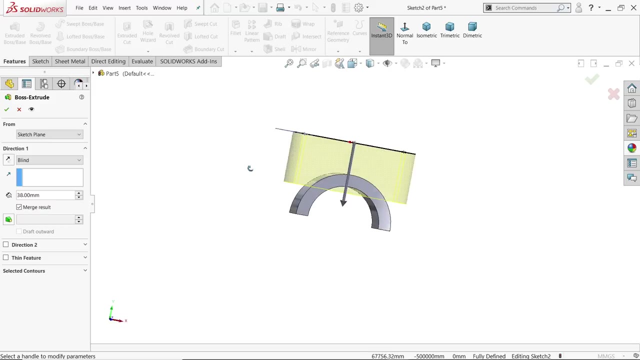 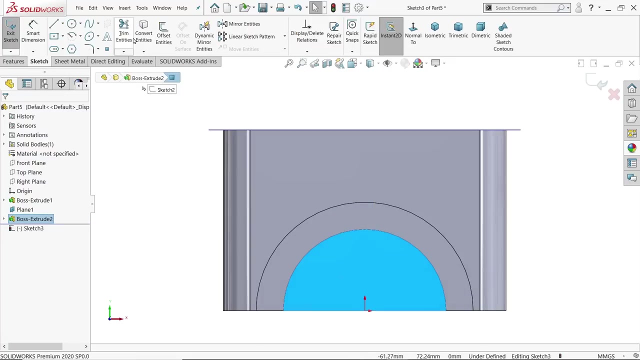 0, 0, 0, 0.. Fritz Her Clark, 01.. Okay, Let's Extrude. This is bigger than this, so we can use only up to surface. up to here, okay, I'll. 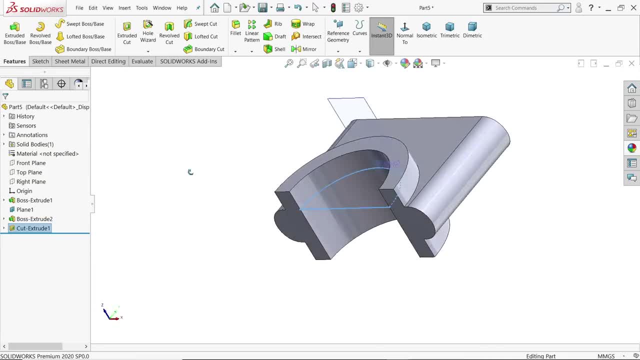 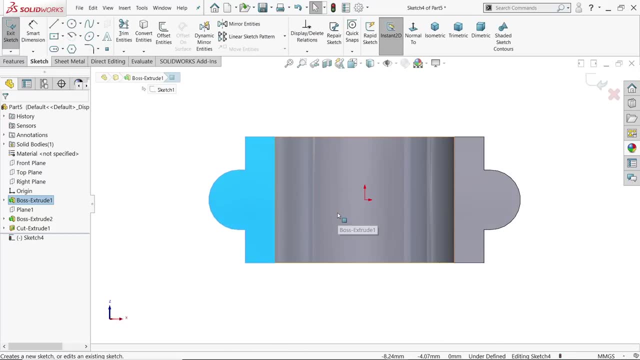 select the face Sketch, Convert entity Feature and select Extruded Cut and simply click through all. let me hide. select this face sketch. now here let's make a whole nine in the same parallel side. even though you can mirror or there are many ways to create this. 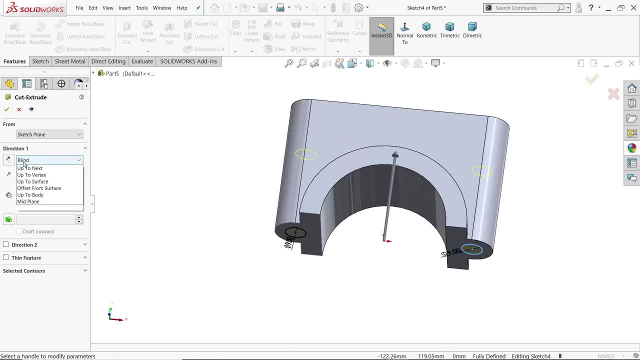 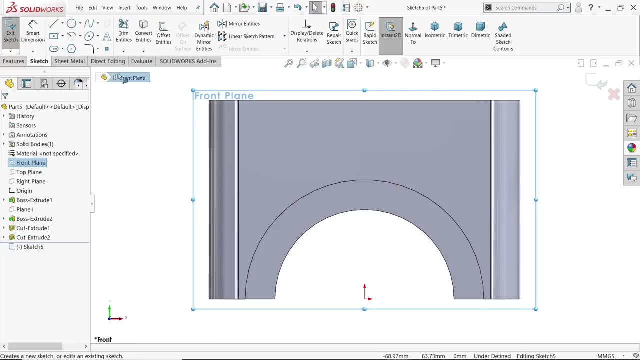 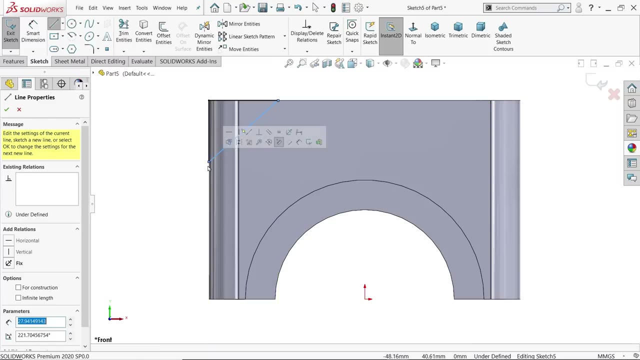 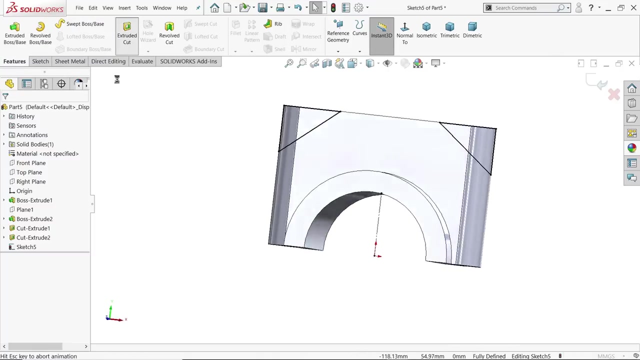 one, but simply keep and condition through all front plane is fish. now here we want to make cutouts. this is seems like this: now make one center line construction line, 20 millimeter, 25 millimeter. now select all lines. mirror entity. it's mirror here extruded cut. 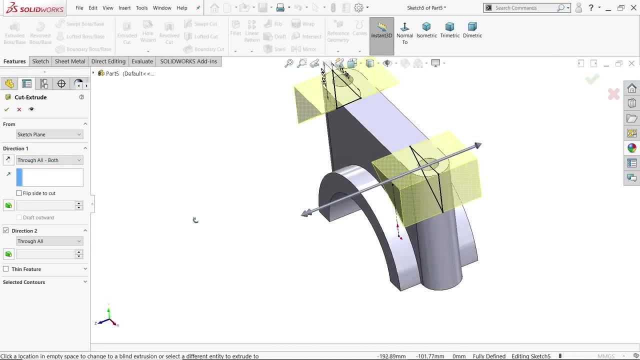 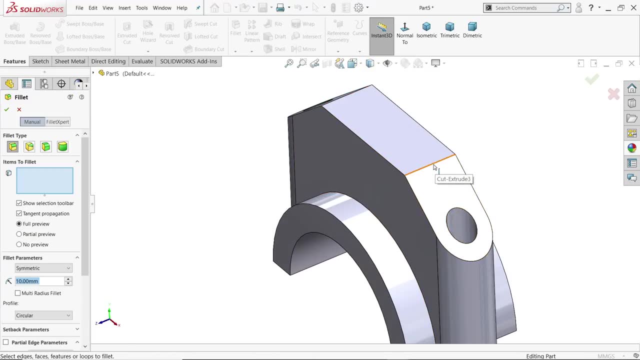 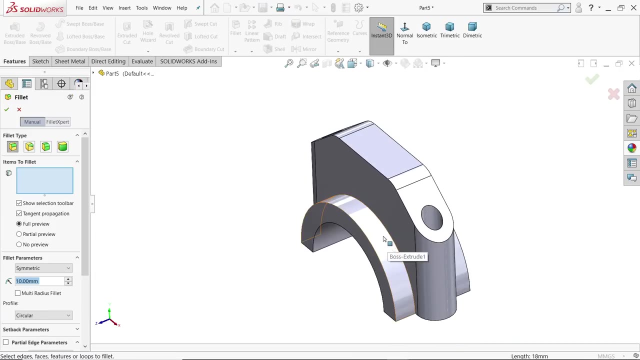 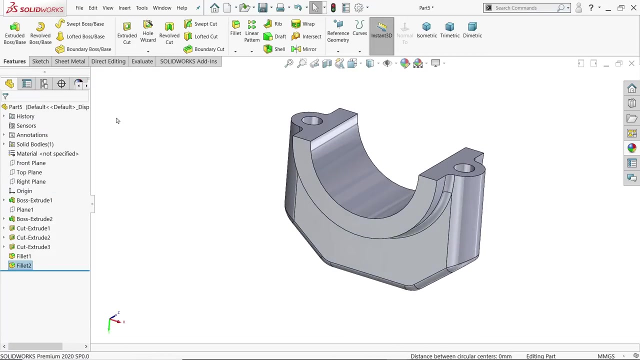 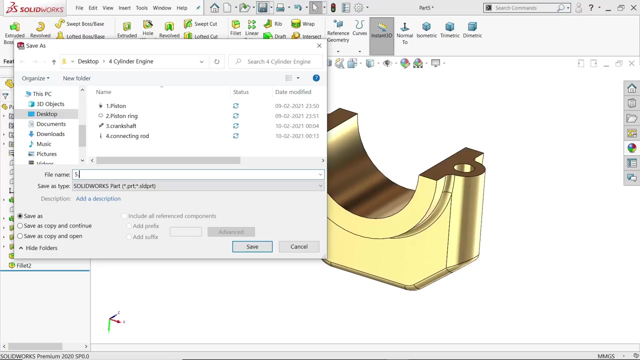 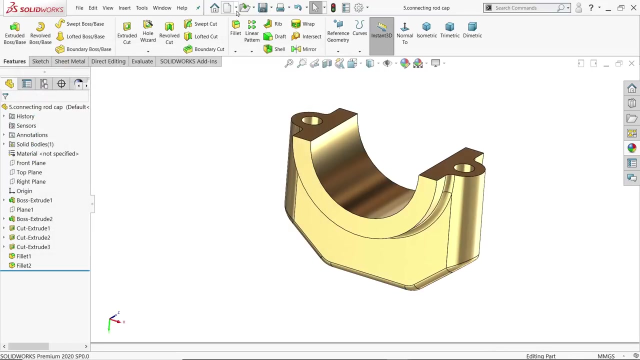 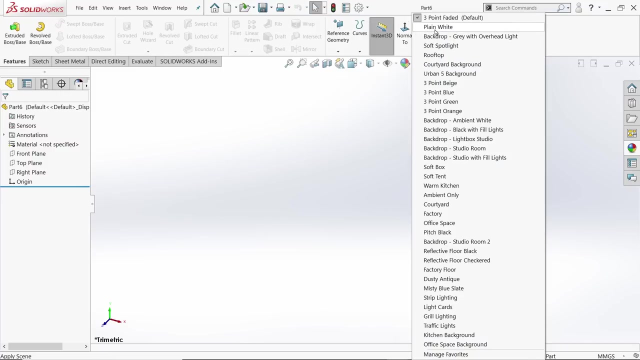 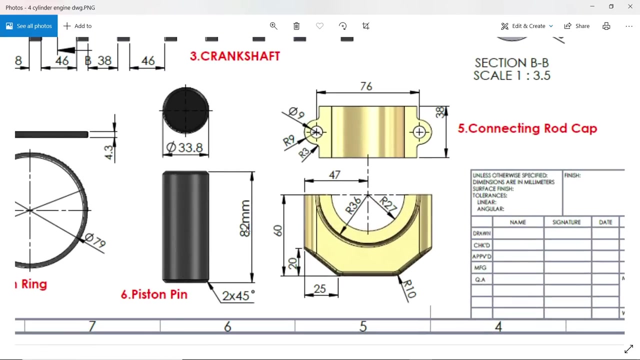 keep and condition mid plane or through all both. see fillet 10 millimeter and choose this tool. okay, again, 3 millimeter, I'll choose one to this age. okay, look again. okay, make lightly, Jess, get 形状. save part number five: connecting rod cap. let's make a new part. the new part is piston pin. it's. connection rod cap. let's make a new part. the new part is piston pin. it's 33.8ollmm, 82mm. the diamonded, the diamonded, the linearsnippet. i'll do righcalculate. currently the diameter going to cross ring tip 110 millimetre. it's above the ring tip 1,1 and 12 mm. 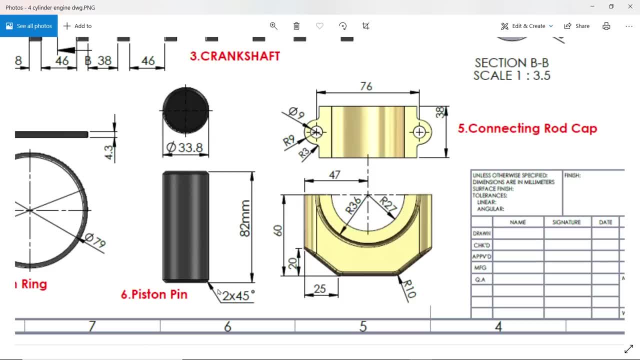 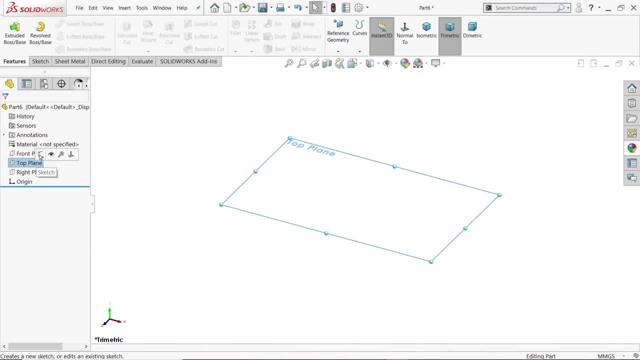 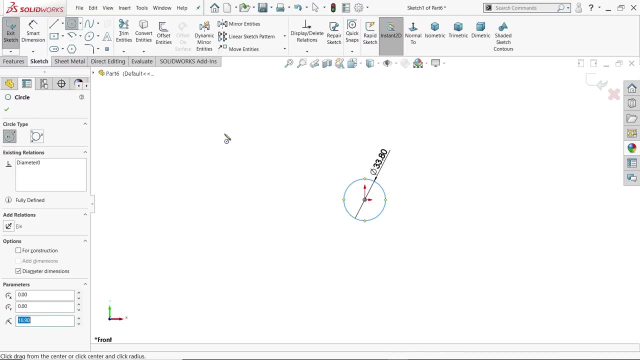 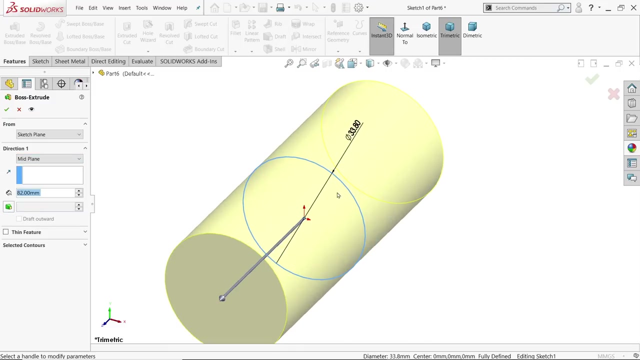 Let' make a new part. the new part is piston pin. it's 33208 millimeter, 82 millimeter the ANY way diameter and there is a chamfer, 2mm 45 degree front plane sketch. draw a circle and that is 33.8, extrude 82. we will keep mid plane because it is very useful during assembly. 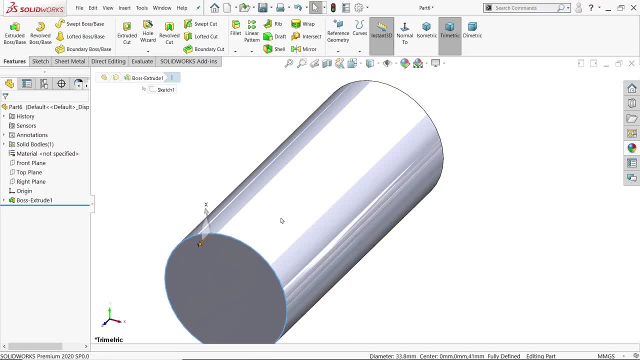 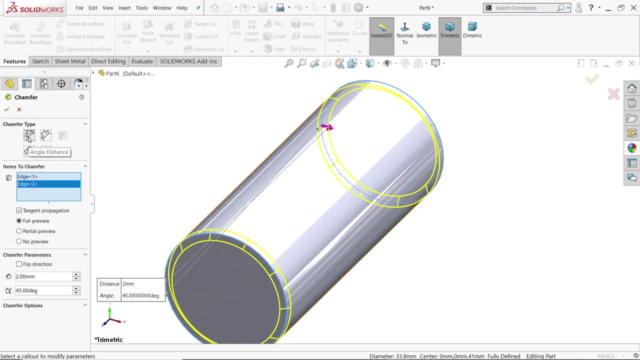 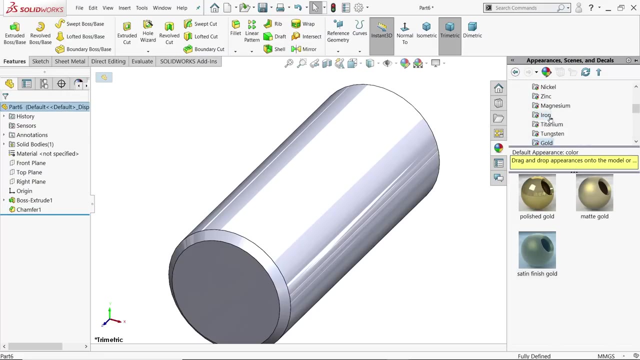 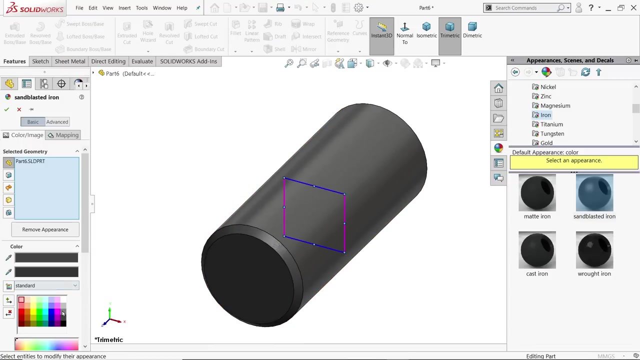 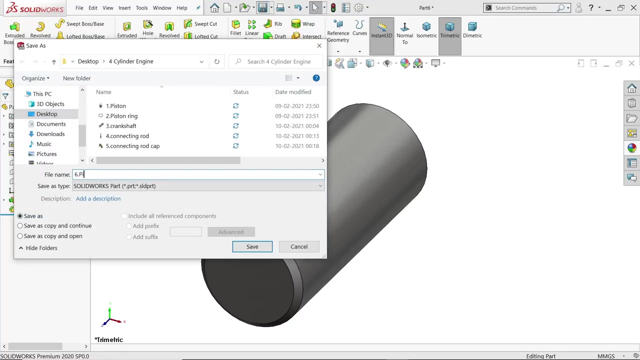 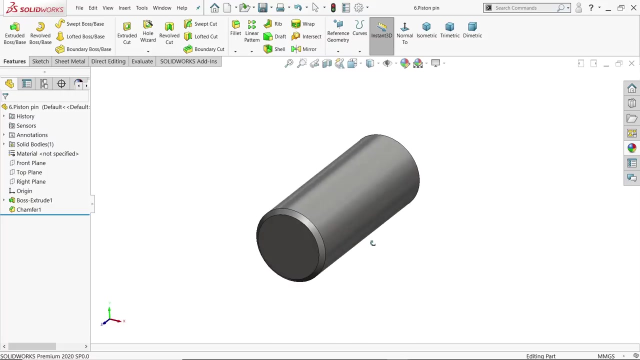 even though if you click on edge you will find option: fillet chamfer 2mm, 45 degree. select other end. we selected angle distance. now piston pin: keep little light, save, ok. ok, piston pin now. now let's start assembly. simply go to make assembly from parts. now first part. 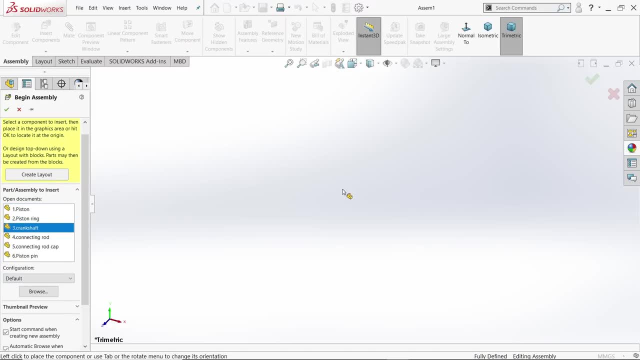 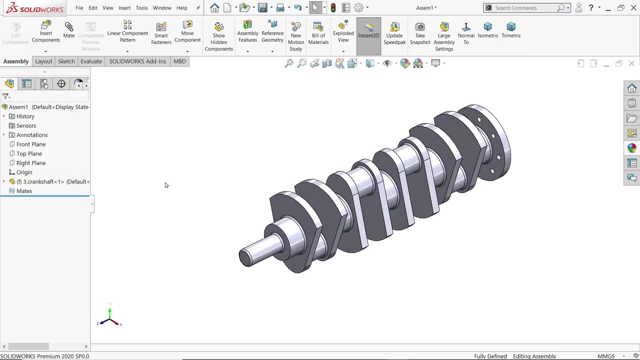 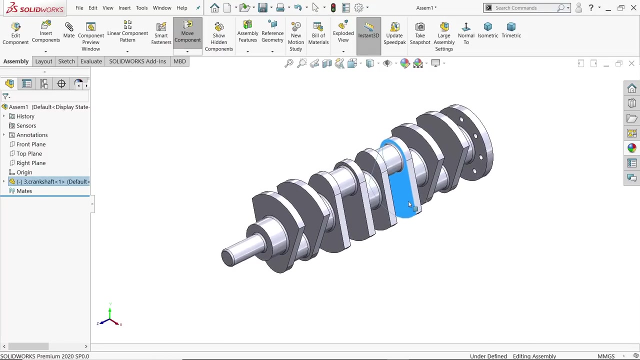 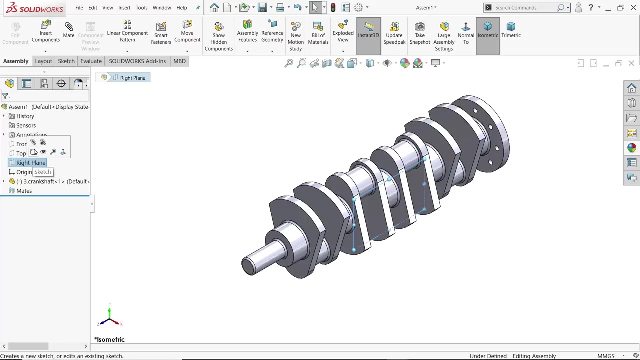 we will bring crankshaft, click here. ok, plane piston. now we want to fix this one first, right click and click here floor so that it will easily move. otherwise it want, if it is fixed, it want move front plane. sorry, right, just makes section right. plane is better sketch. let me draw the. 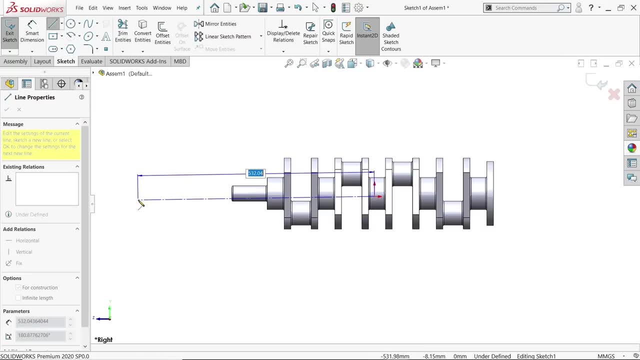 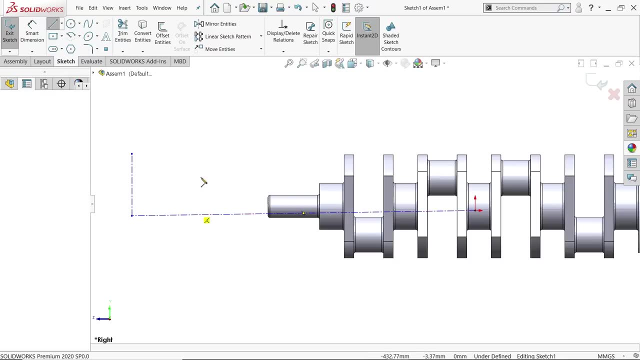 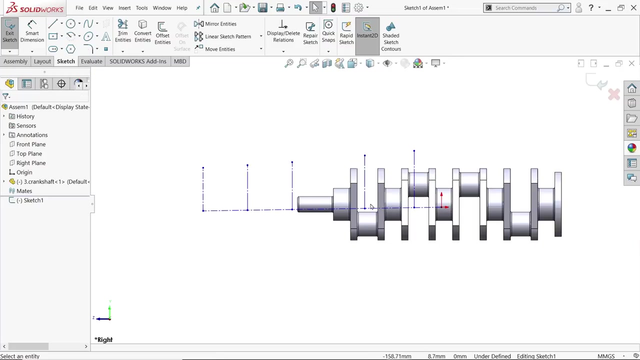 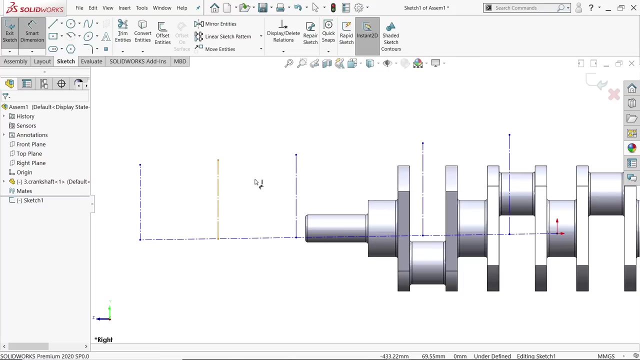 line is scattered. ok, ok, this is very useful. this is actually our path. again, select line, escape L key on keyboard and you can draw a line. escape again L key and draw a line. now select this. all lines make symmetry. let's define dimension hundred and fourteen. this is the distance between two piston and we are. 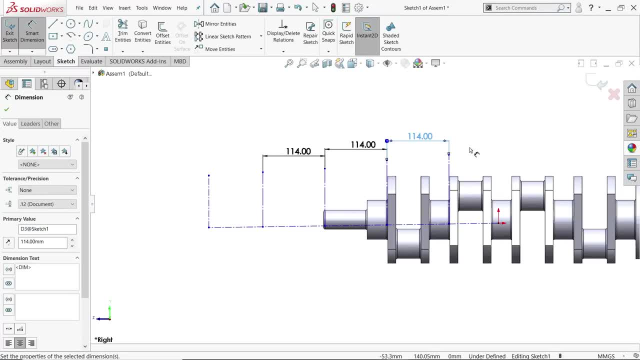 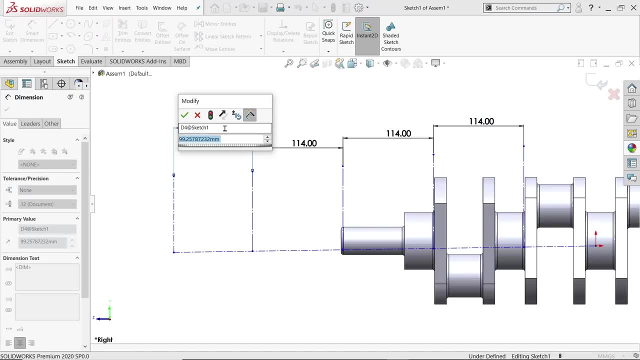 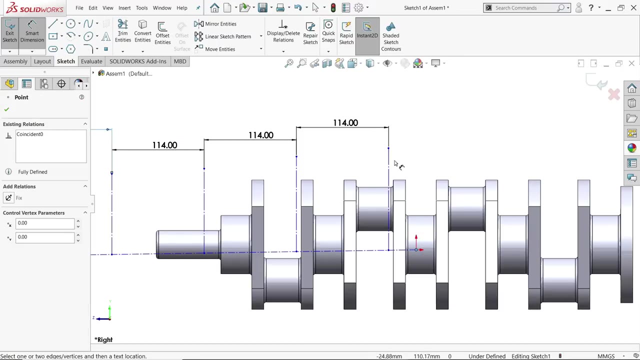 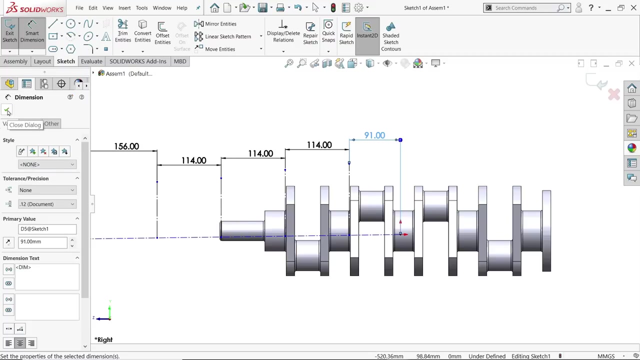 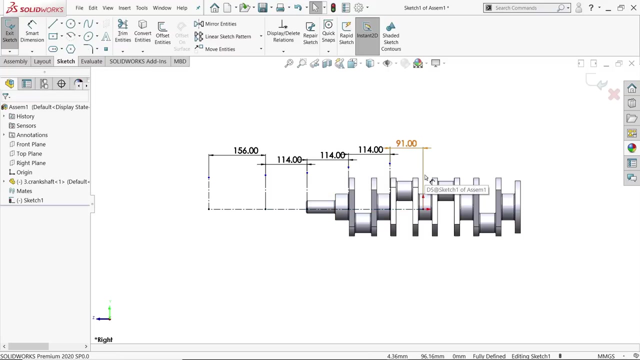 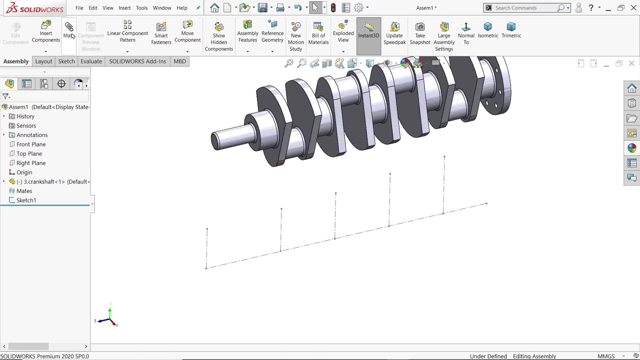 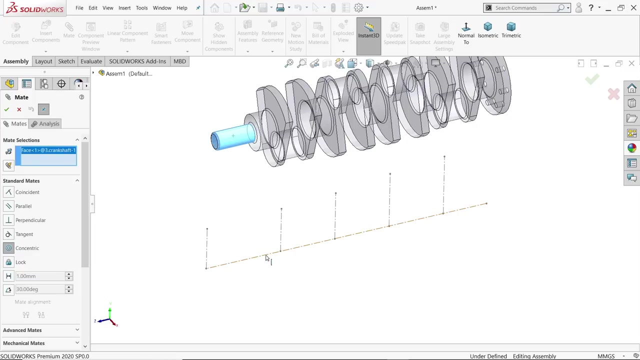 going to fix this piston. now make distance from here to here: 91, this is the distance from this end. okay, this is not seems fully defined. okay, make horizontal. now this is fully defined. sketch exit: it is moving like this: let's make a mat concentric. select this one because this is the center, and this one, okay now. 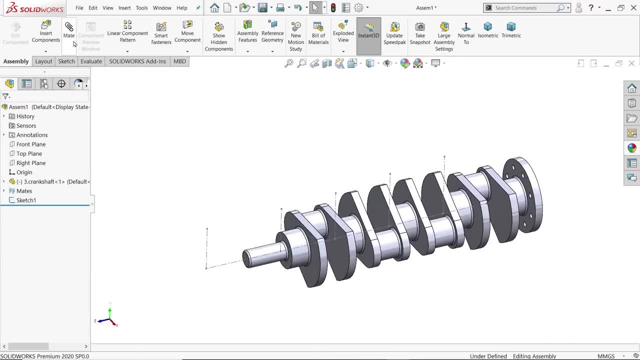 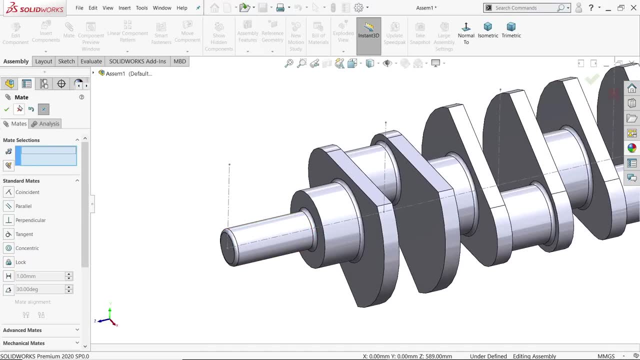 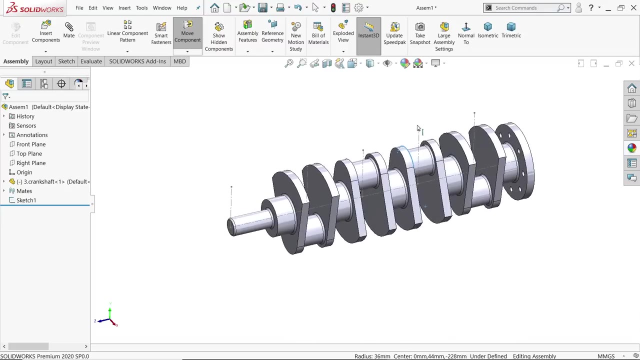 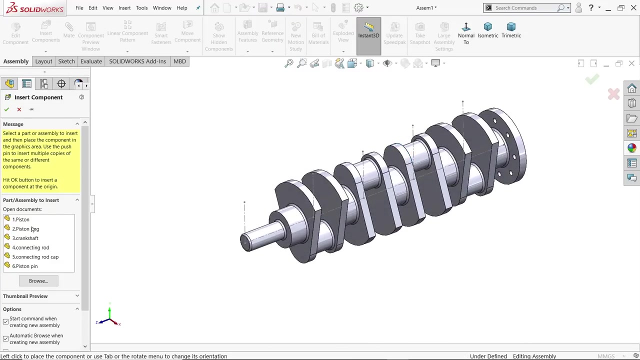 let's rotate. see, it is going to rotate with this. the last relation, this end point and this face coincide relation. okay, exit. now let's say: okay, look, it's rotating like this. okay, this is the our position. insert now control key one, two, three, four and let's insert piston pin. 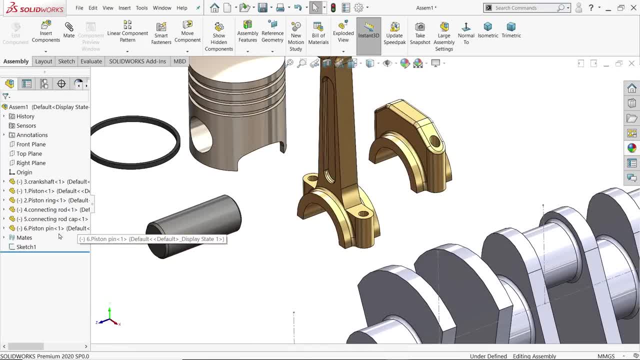 okay, this is our position. insert now control key one, two, three, four and let's insert piston pin mat first, piston front plane of piston. come down piston pin, hold ctrl key, front plane of piston pin and here you will find option. mat see is going to coincide. entry is going: 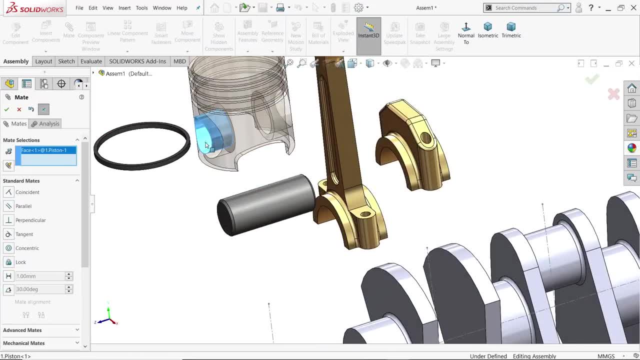 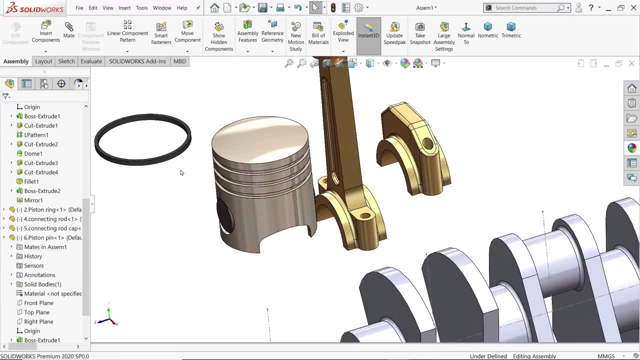 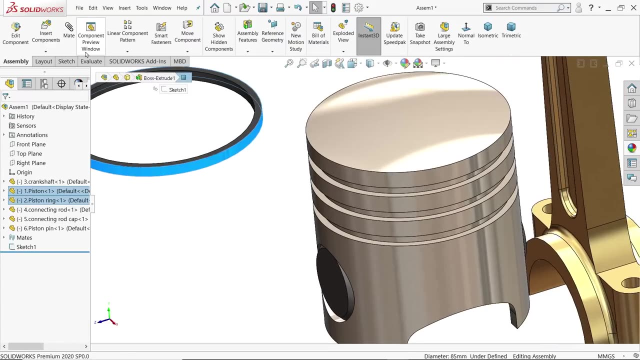 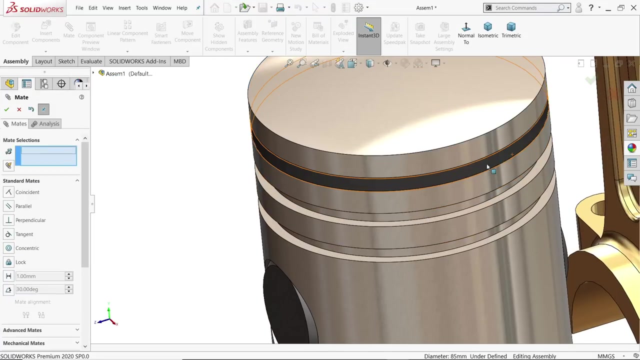 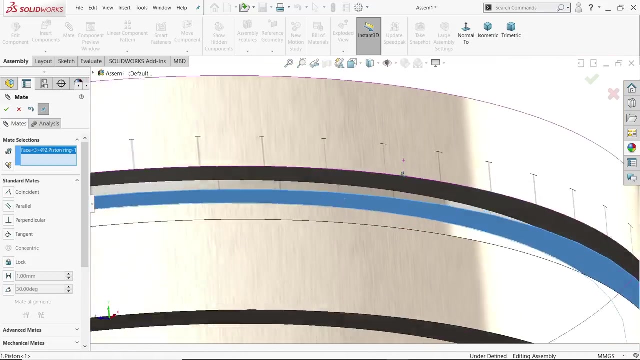 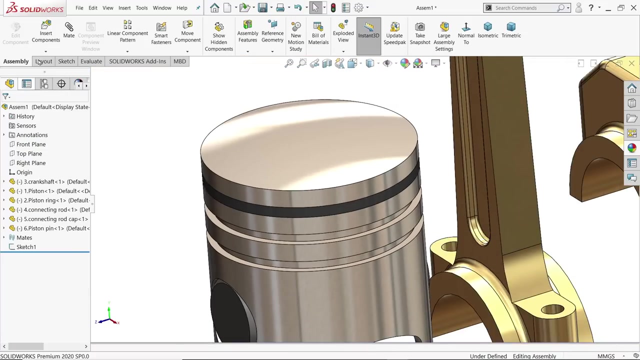 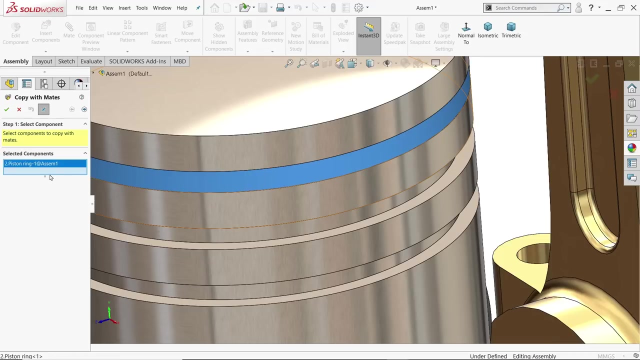 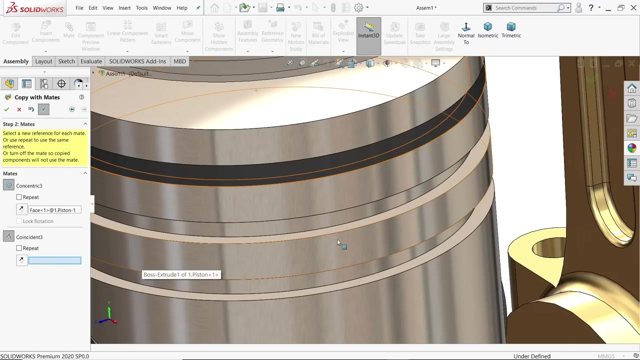 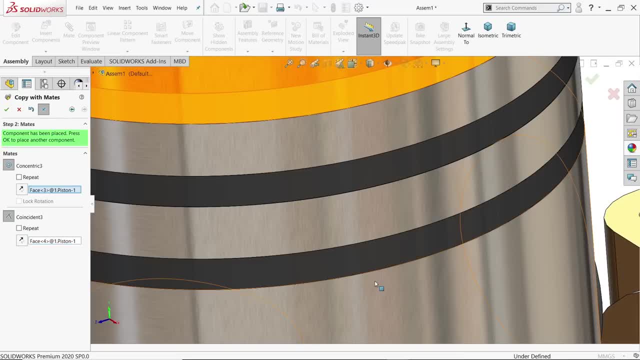 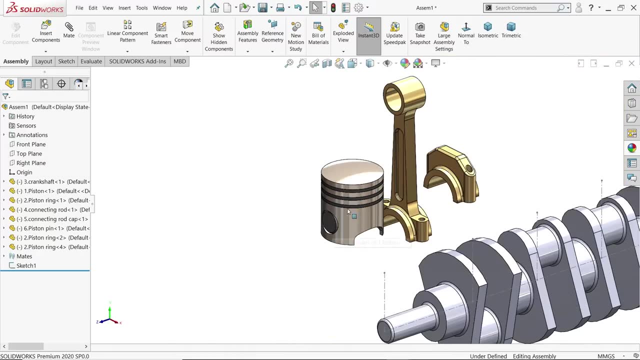 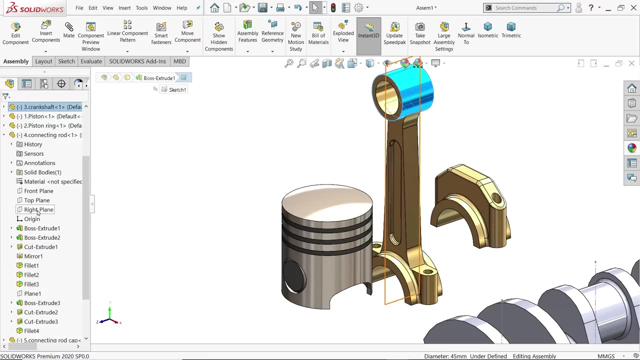 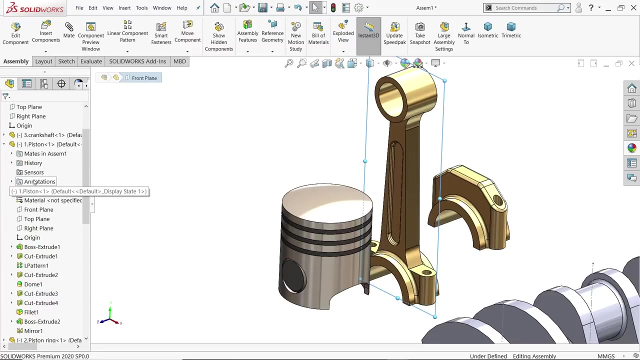 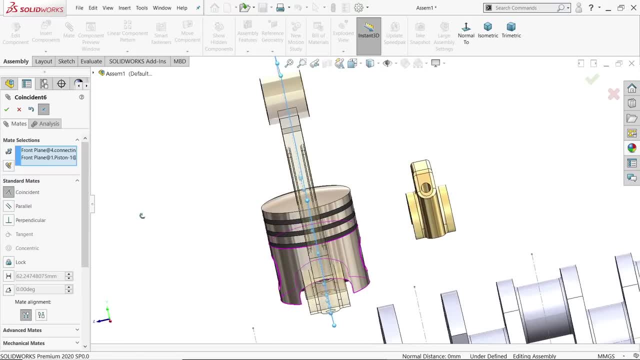 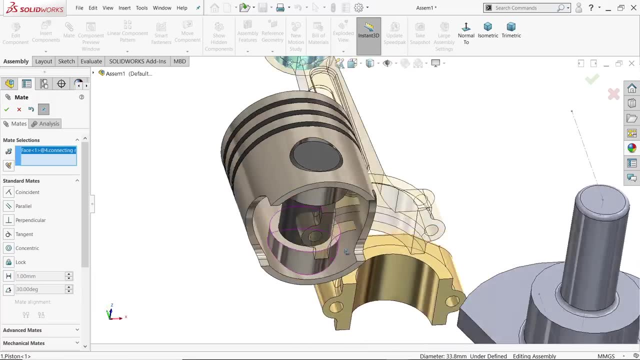 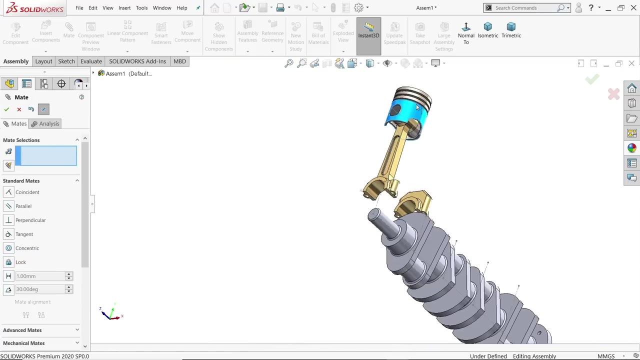 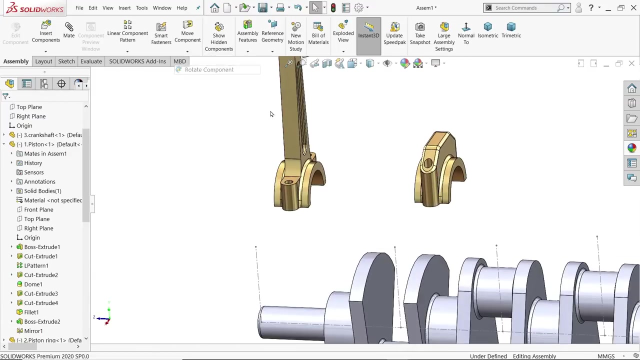 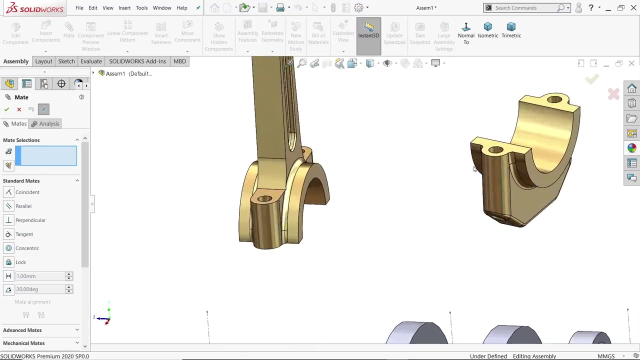 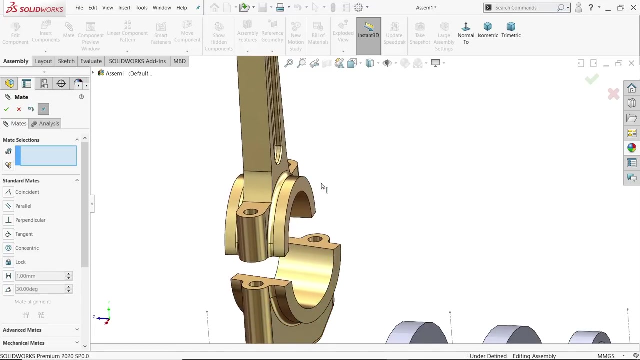 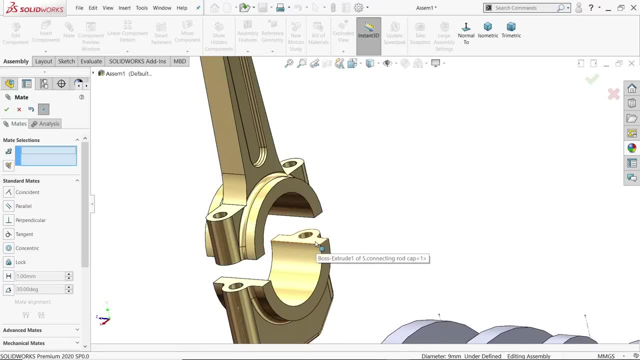 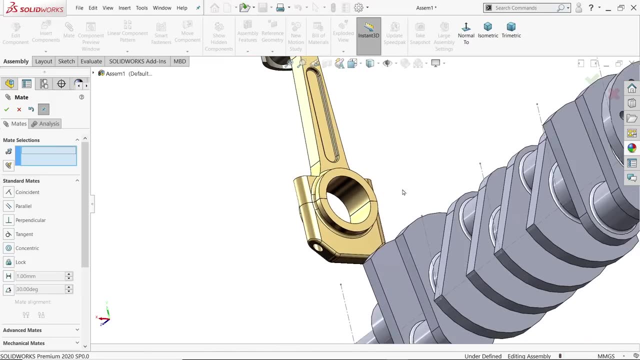 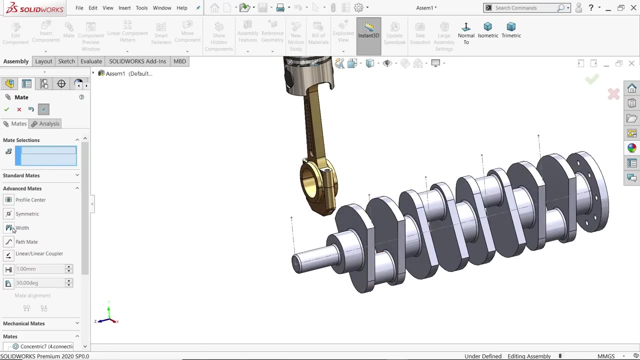 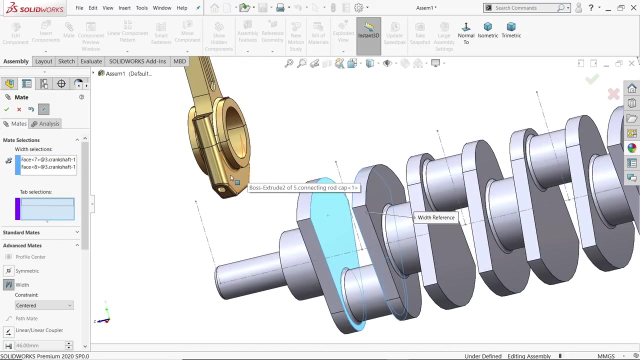 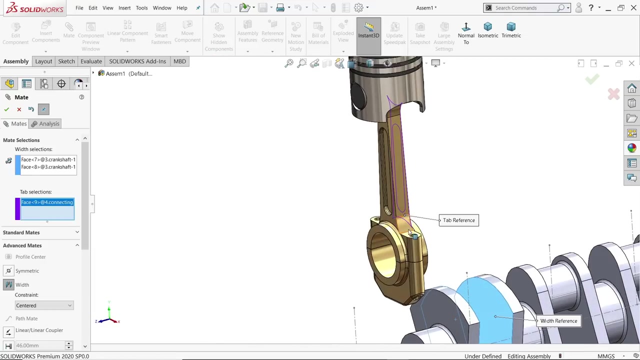 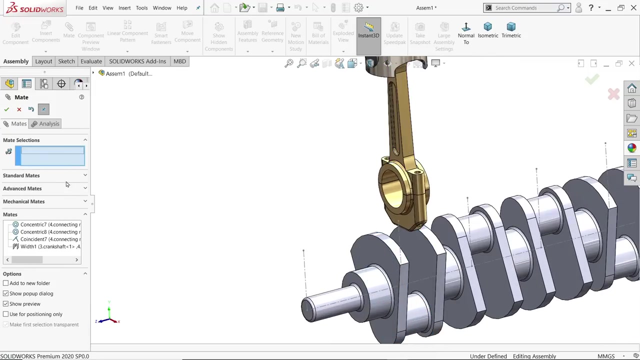 hole go. centric relation: this face, this face coincide relation. okay, now we we are, we need to fix here. so there is one option called advanced met, width met. I will select one second to face or any two face of this. okay, but one important relation we forget, oh, centric relation, this one. 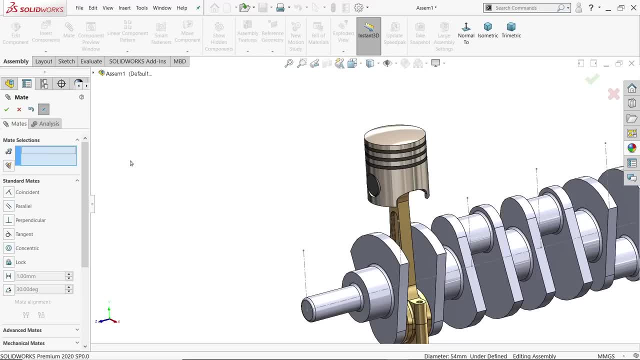 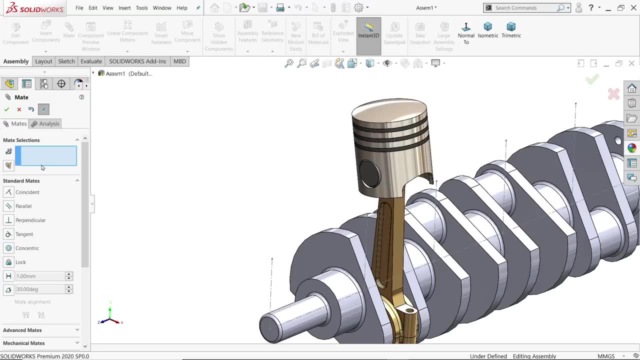 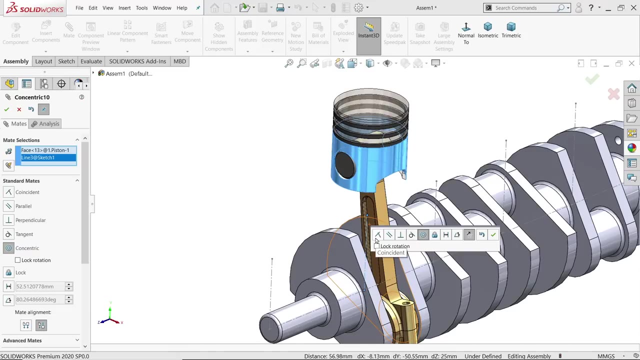 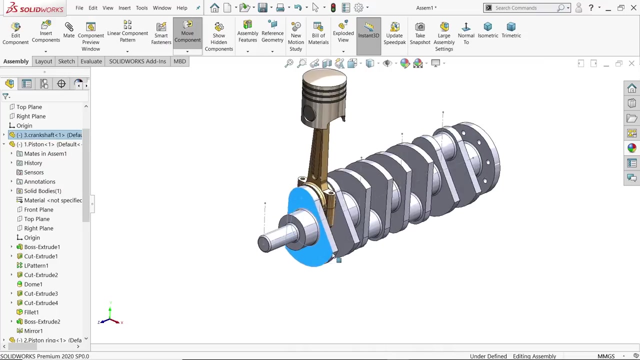 and this one co-centric relation. okay, now one more a important relation. see, it is moving like this piston body and this line co-centric relation. don't make coincident co-centric relation. okay, now i'll show you how it's going to move. look, now we will use copy mat command. 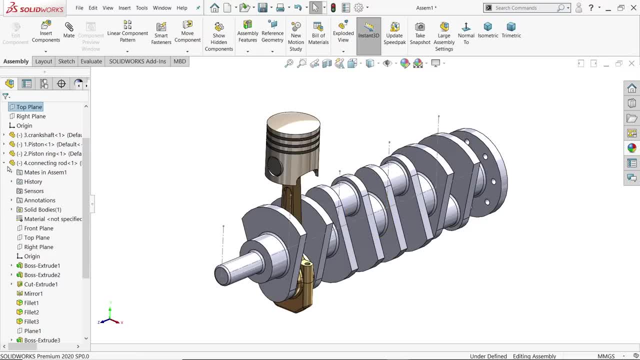 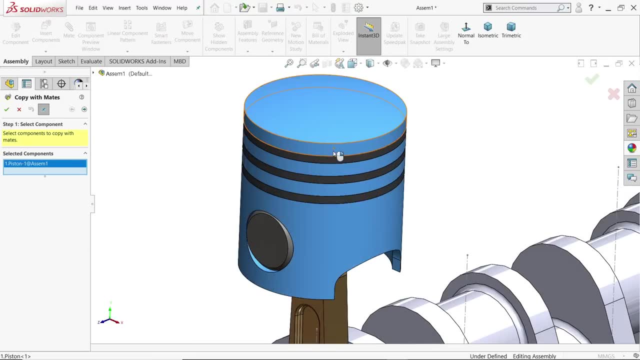 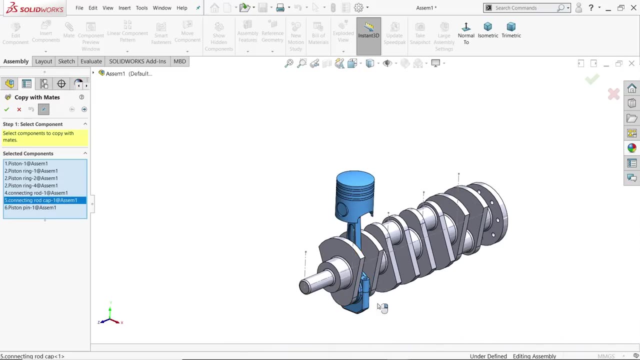 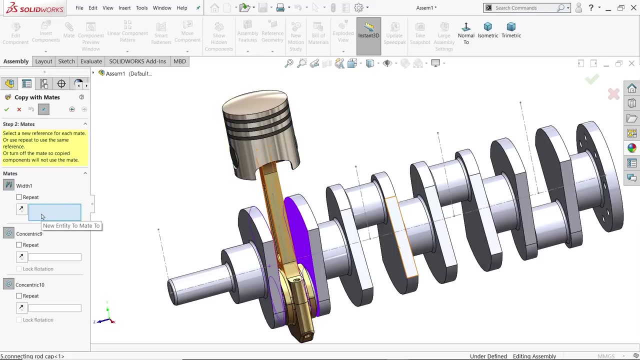 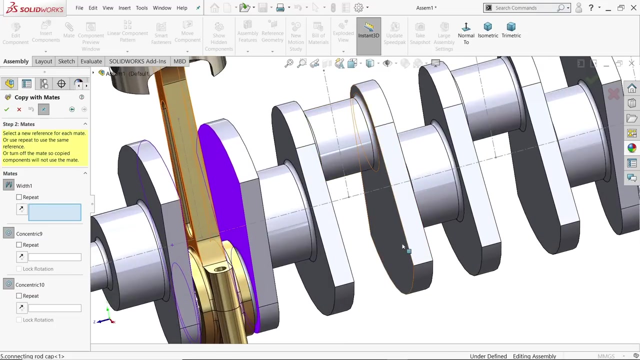 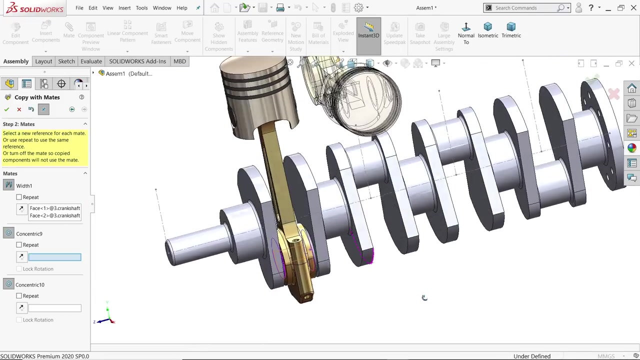 let's hide copy with mat. now here i'll select all component: one, two, three, four, pin this one and this one. see, i'll select next. now i have to choose width. so for width, we are going to fixed here, so i'll select one, two. okay, now the next option called co-centric. so i'll select this one. 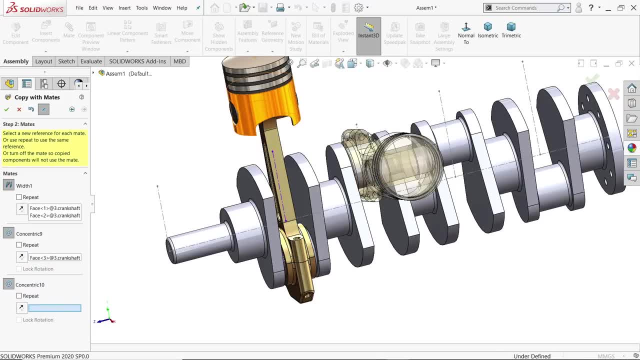 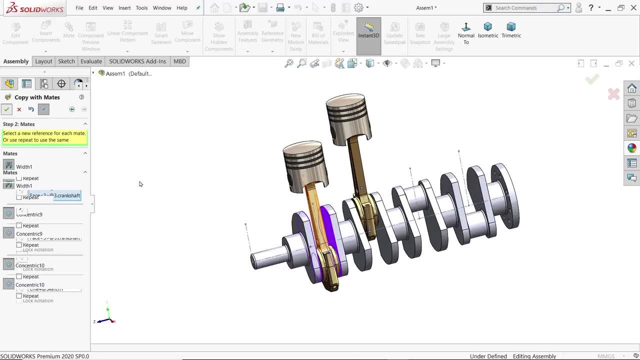 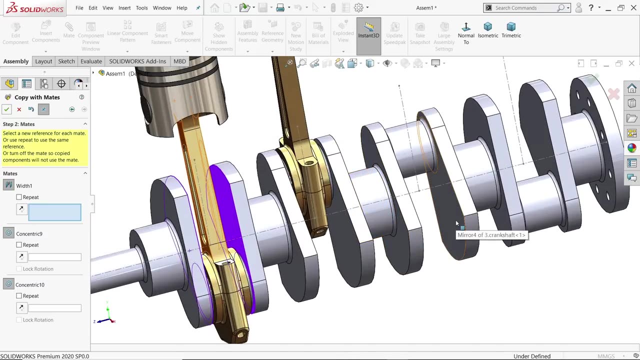 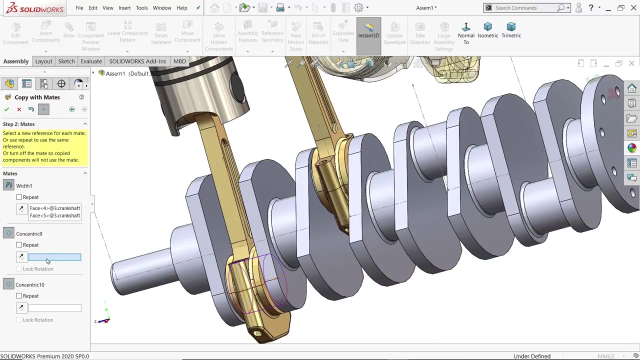 okay, the next option, again co-centric, so i'll choose this line. look, it's going to fixed here. okay again, width: ok, one, two now co-centric for this and the third one co-centric for this line. this is checked very careful. this is very important tool because it says: 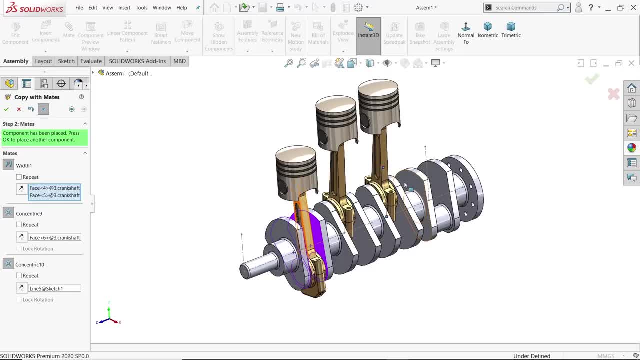 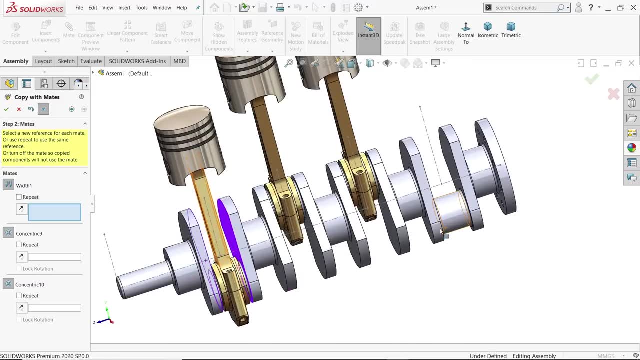 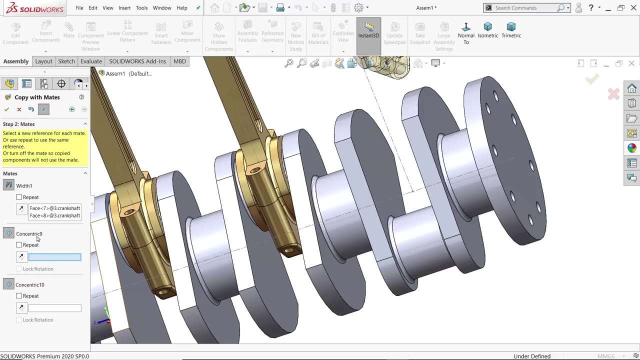 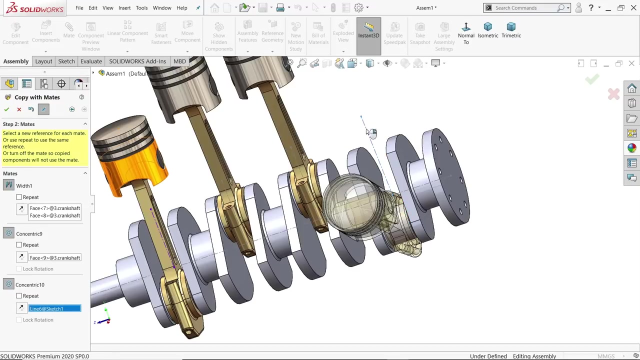 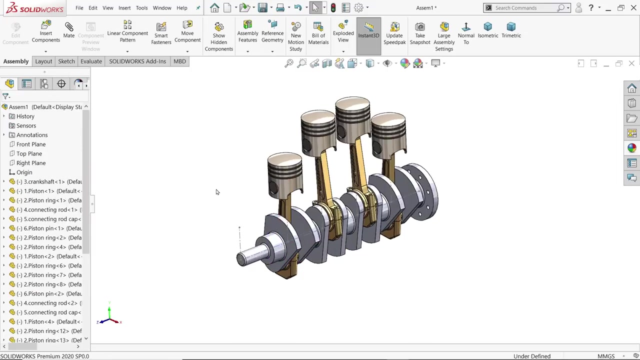 your lot of time, otherwise you need to fix one by one, each and everything and it takes too much time. say yes again. we will apply the same thing to first width command. so one face, one face to now: co-centric relation this rod. co-centric again: relation this line: okay, cancel. let's check, rotate, see fixed. 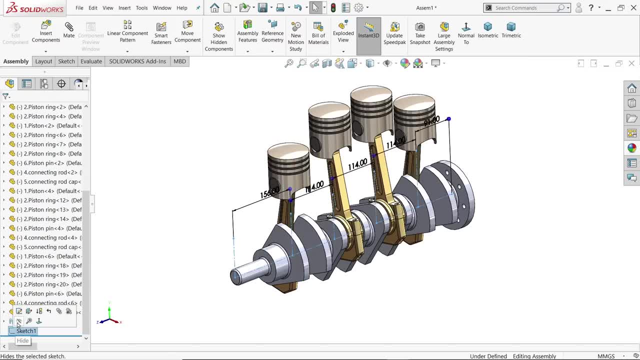 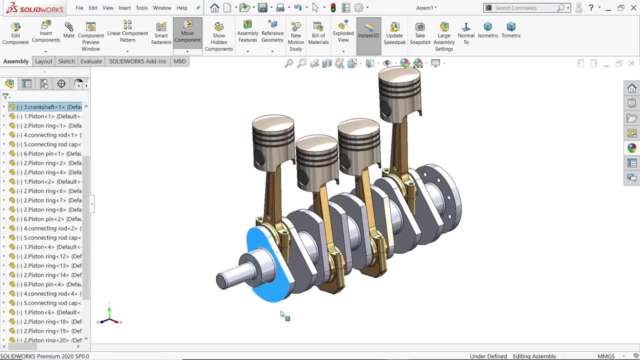 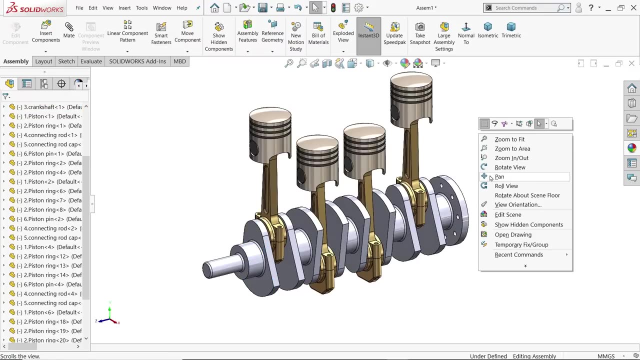 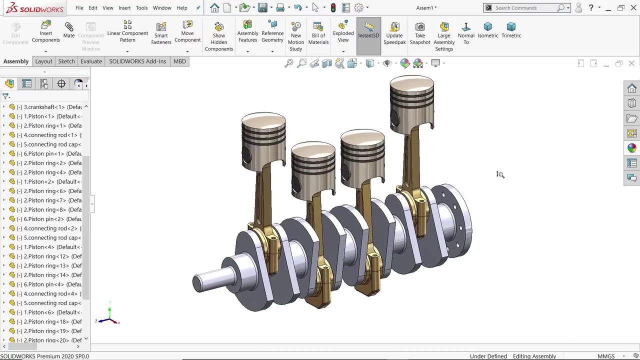 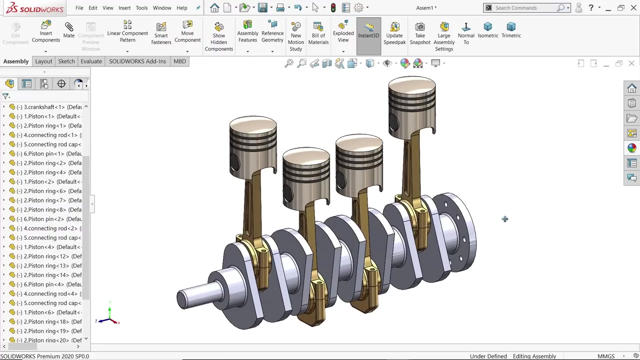 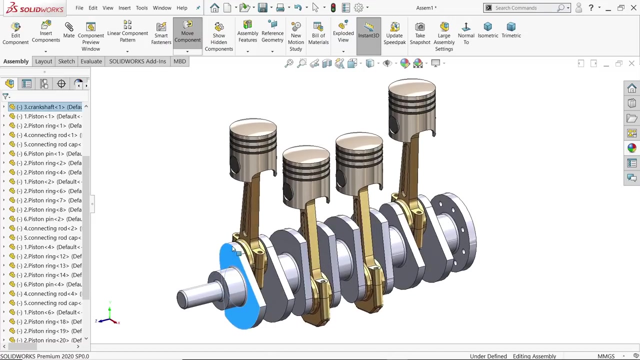 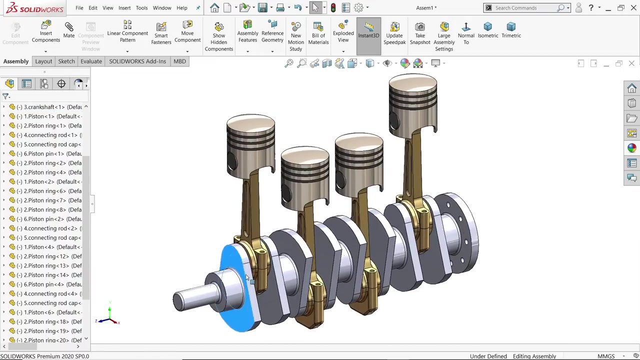 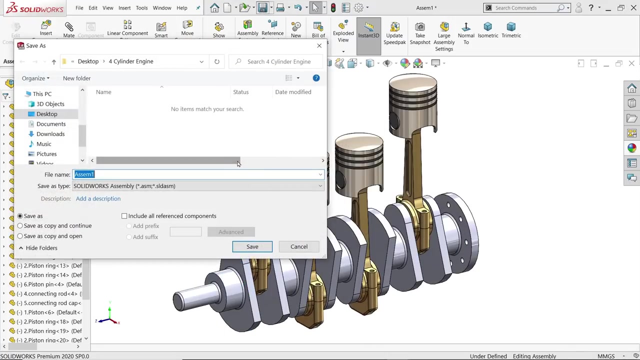 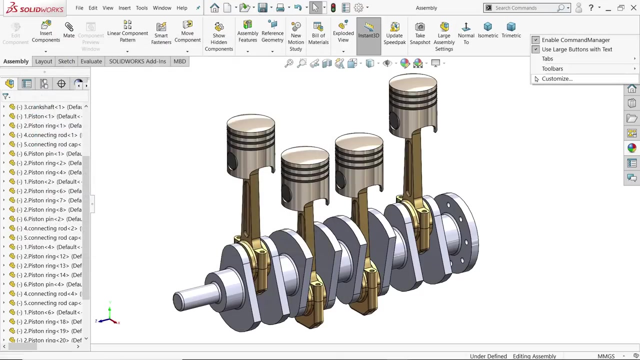 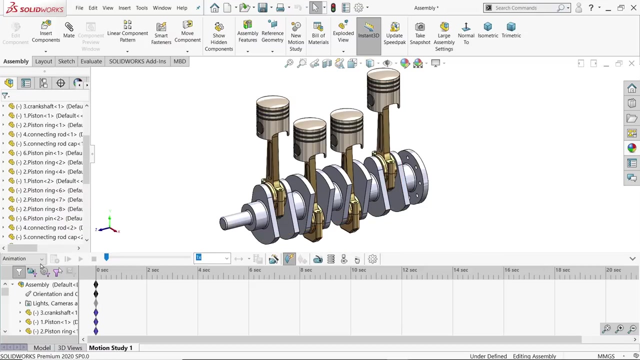 now I'll hide. okay, this one seems perfect. let's make a proper location, okay, let's make little bigger. let's rotate, okay, even though still there is a possibility. okay, that's fine. let's save this one as a assembly. now right-click to motion manager, go to motion study. keep your basic motion. I will select frame. 50 frame seems to be fine. 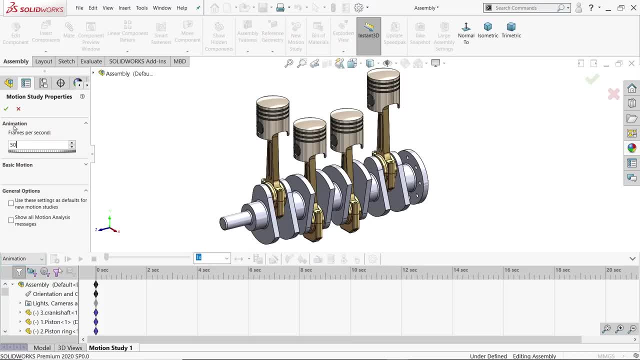